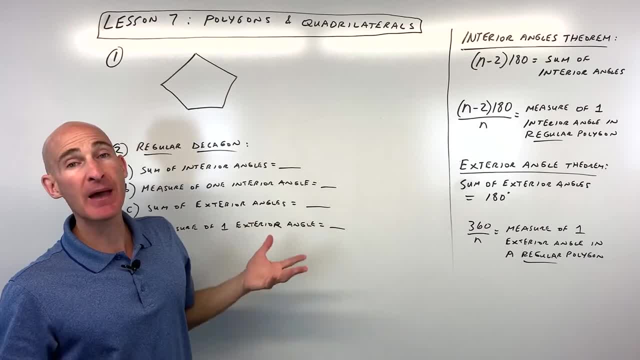 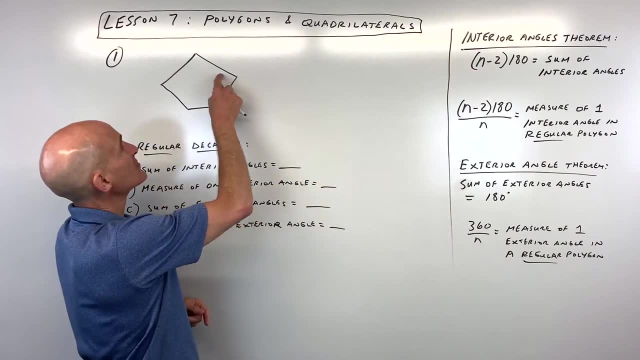 So, for example, here you can see, we have a polygon. specifically this is a pentagon because there's five sides: one, two, three, four, five. But when we talk about the measure of the interior angles, these angles here on the inside, what we can do is we can use this formula here: n minus two. 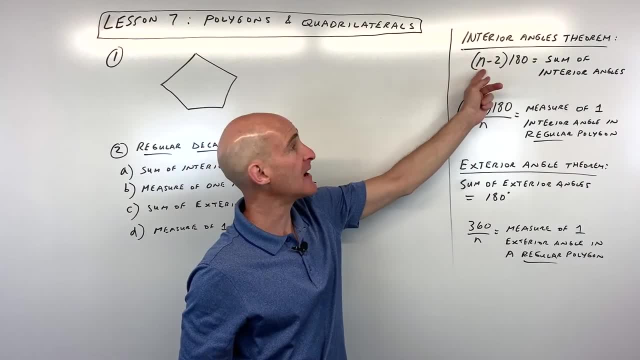 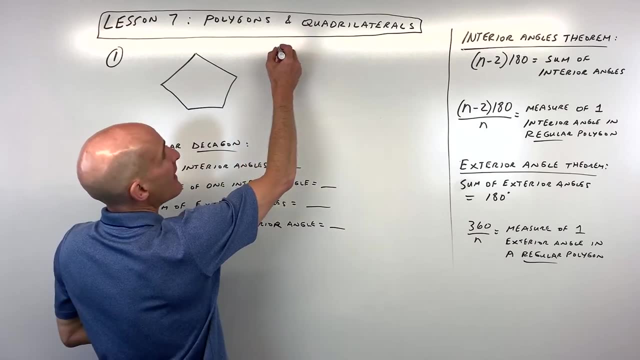 times 180 equals the sum of the interior angles, where n is the number of sides, or you could say n is the number of angles, because they're the same. So for example, here we could say five minus two, which is three times 180.. 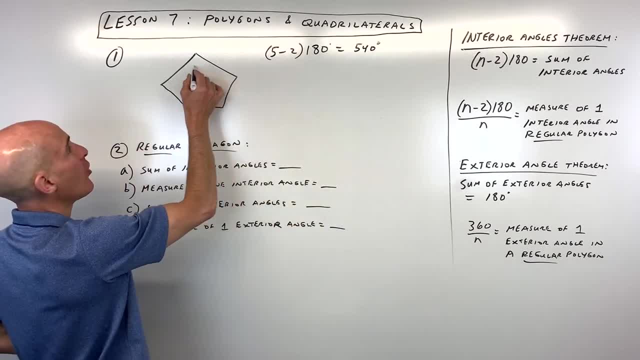 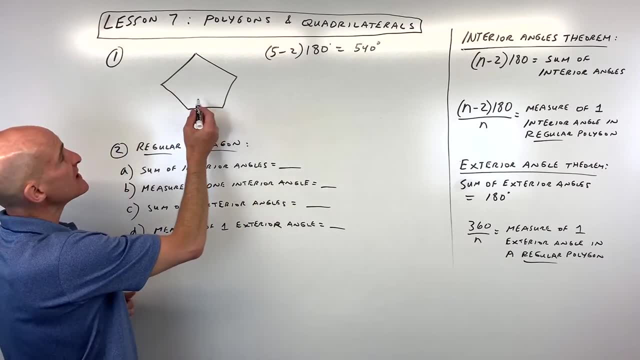 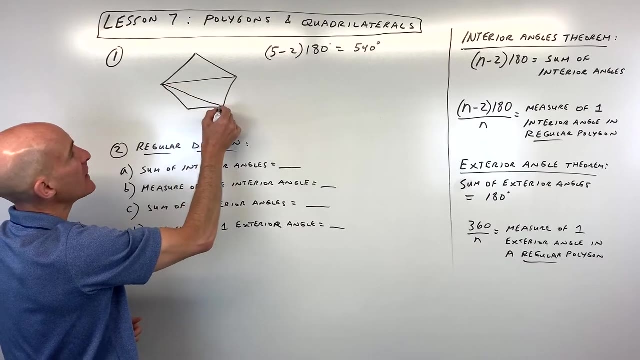 That's 540 degrees. So that would be the sum of all these interior angles. Now, they don't all have to be the same measure, they could be different measures. But what you can see is, why does this formula work? Well, we know, in a triangle, all the angles add up to 180 degrees. right, And you can. 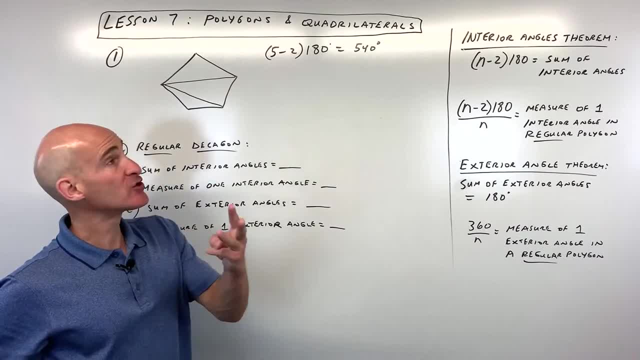 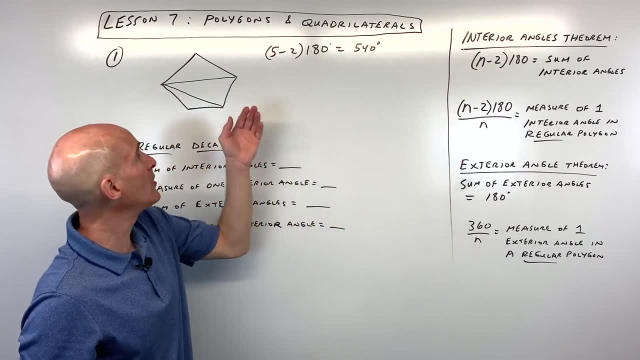 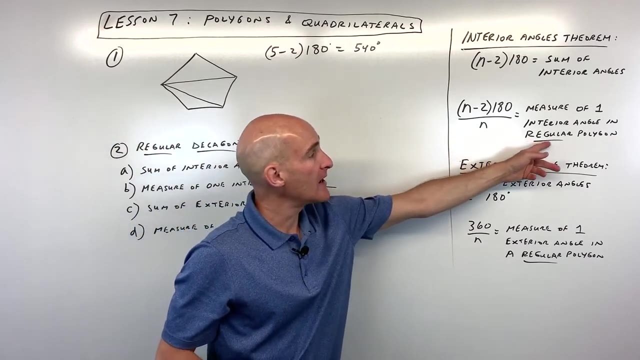 see, we can subdivide this pentagon into three triangles, two less than the number of angles right. Five minus two is three. there's three triangles: 180 degrees in a triangle. that gives us 540.. So that's where the formula comes from. Now say, for example, it was a regular pentagon, or 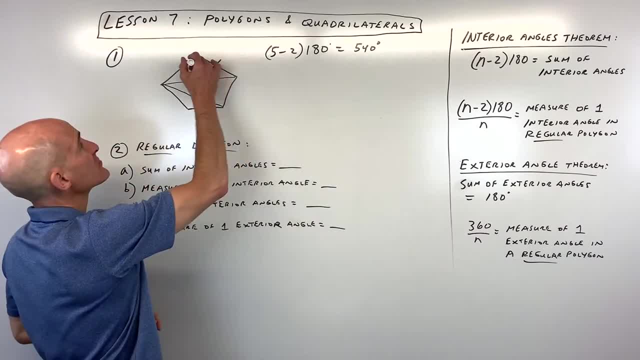 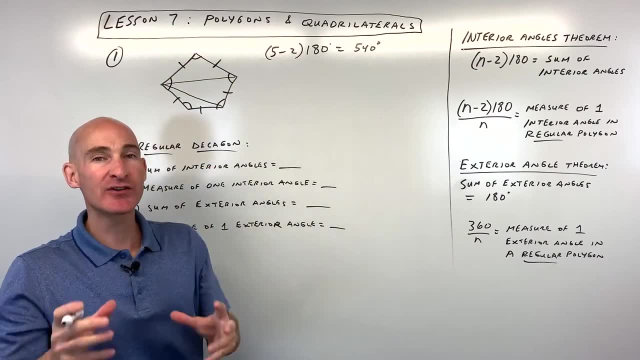 a regular polygon. Regular means that all the sides are the same length And all the angles, these interior angles here are the same measurement. So it's very symmetric. It's what you think about when you think about a pentagon or a hexagon. it's very symmetric and regular. But what you can do here is 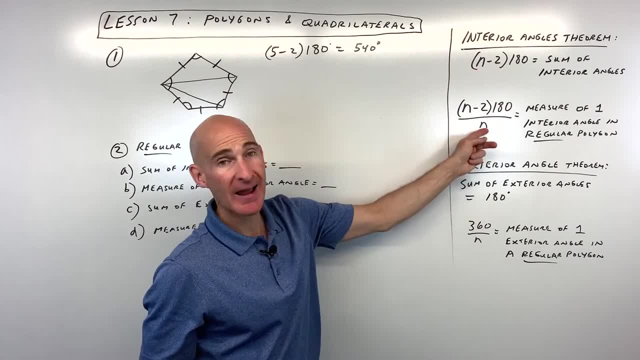 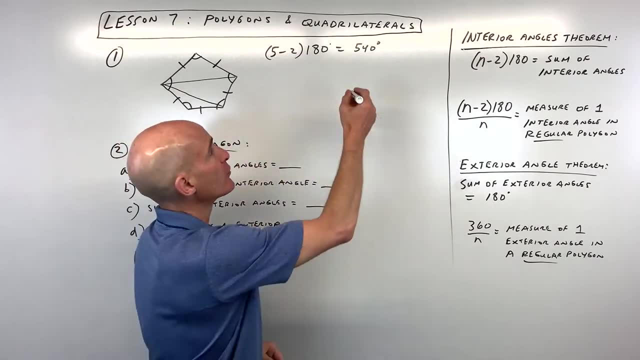 you can take the same formula we use. the only thing you're going to do is you're going to divide by n, which represents, you know, the number of angles, or the number of angles, and you're going to use the number of sides to find the measure of just one of the angles. We know the total is 540.. If we 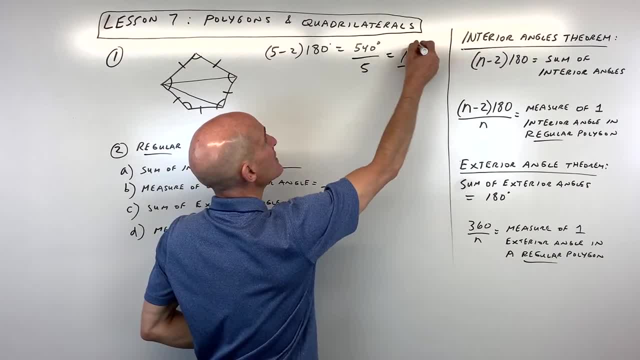 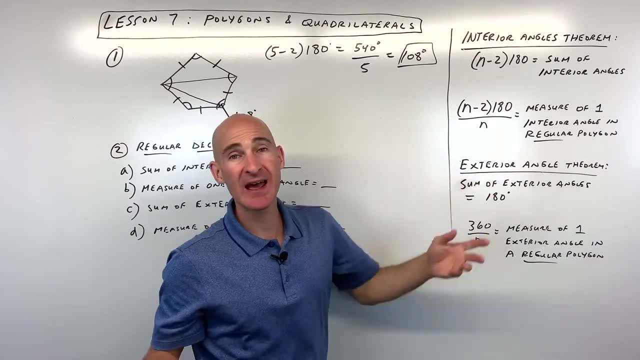 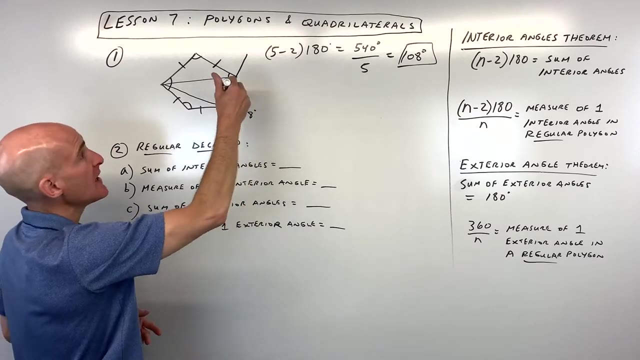 divide by five, that comes out to 108 degrees, And that would be the measure of just one of these angles. Okay, now switching gears to the exterior angles. what's an exterior angle? Well, if you take one of these sides and you extend it, either this one or this one, it doesn't matter which one you. 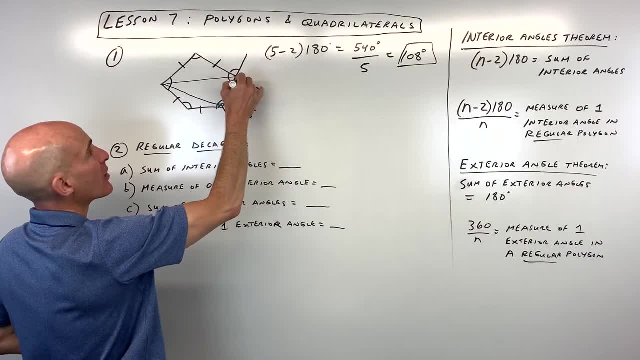 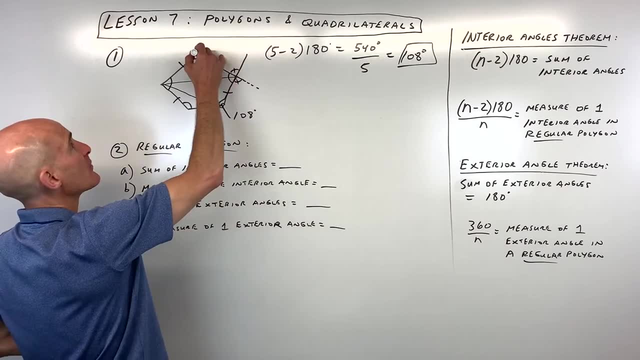 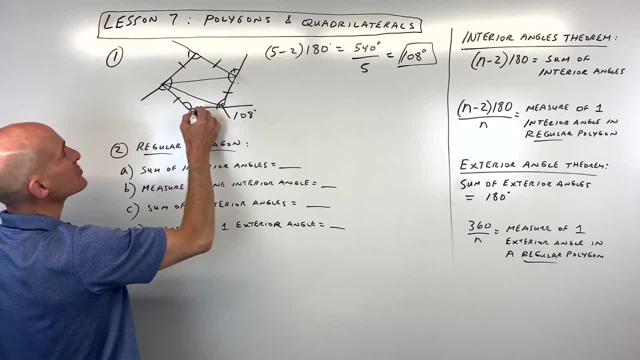 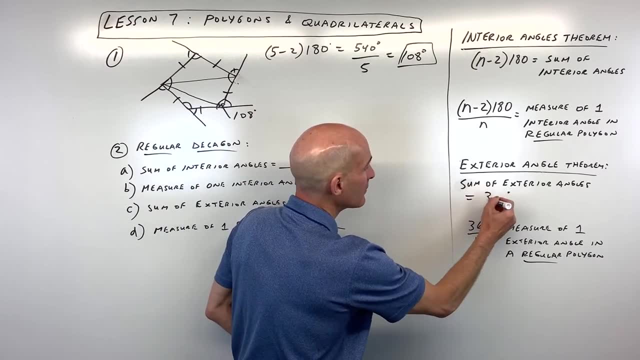 here. So now, if you add up all of these exterior angles, these ones on the outsides, they're always going to add up to not 180, but 360 degrees. okay, just like a circle. So what you want to do is if 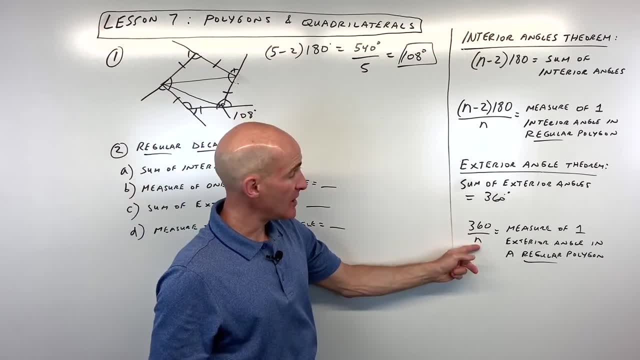 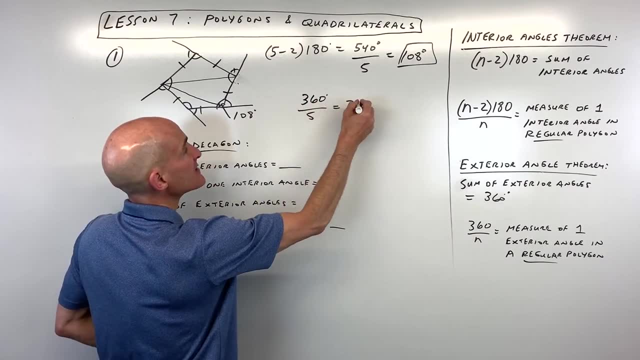 it's a regular polygon, meaning all the angles are the same. you could take the number of exterior angles. take 360 divided by, in this case, five, and you're going to get 72 degrees. Now, one thing that you'll notice is that, see, here's an interior angle, here's an exterior. 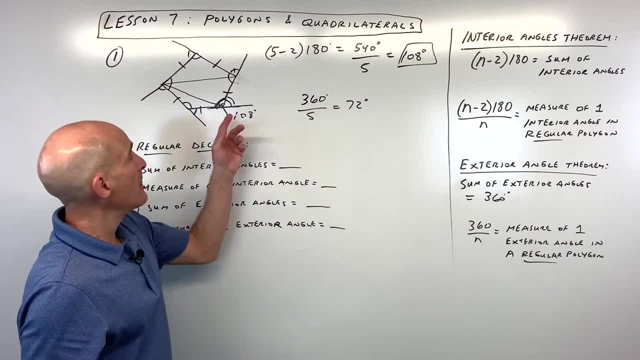 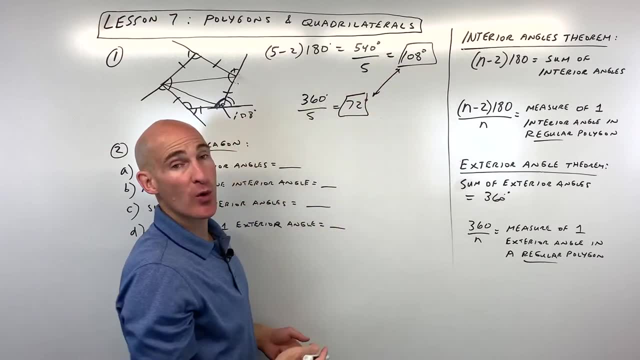 angle. see how they form a linear pair or a line. we know that a linear pair of the angles add up to 180.. And look what we have here. we have 72 for the exterior, 108 for the interior. those add up to 180.. 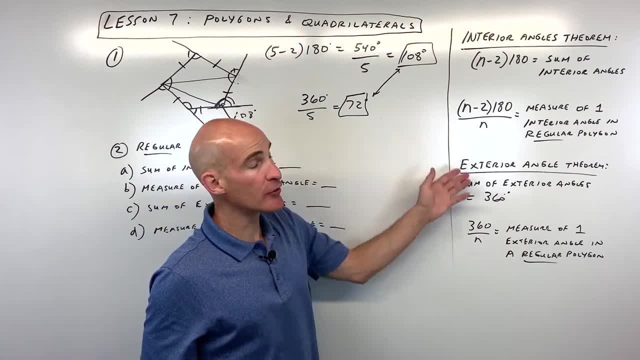 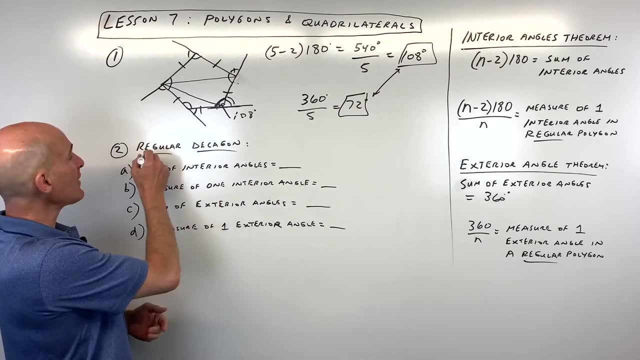 So if you know one, you can find the other one without having to use the other formula. But these are good to memorize or write down on a formula sheet. Let's look at another example. See if you can do this one Here. what we're talking about is a regular decagon, So remember a decagon that. 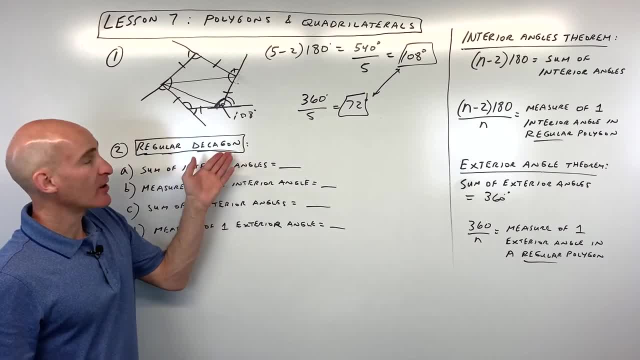 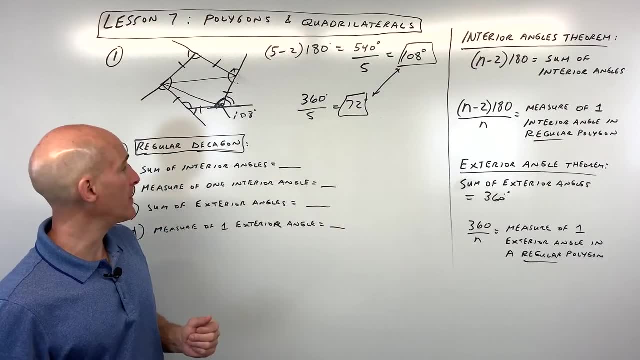 sounds like decade, with like 10 years. Decagon means that there are 10 angles or 10 sides and in this case, because it's a regular decagon, all the sides are the same length, all the angles are the same measurement. So see, if you can do this one, how would you find the? 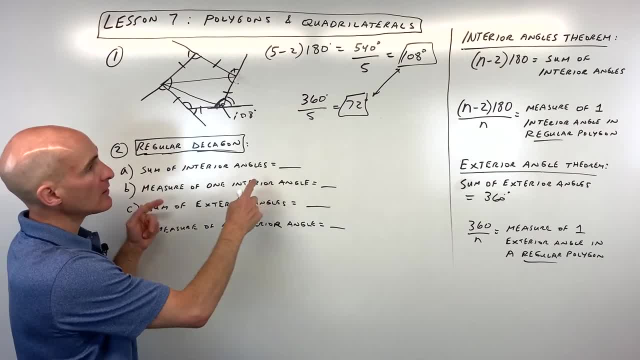 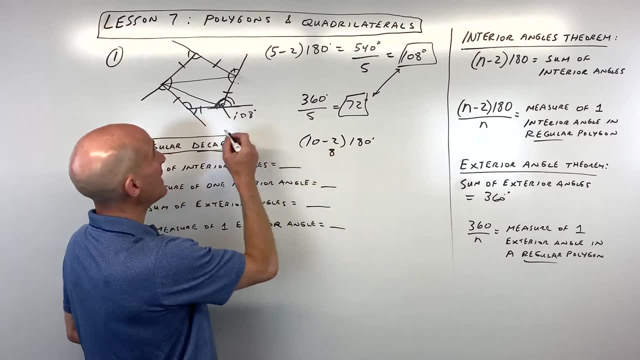 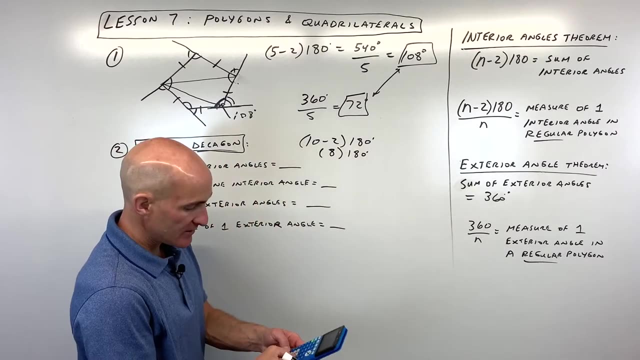 sum of all the interior angles. Well, we can use this formula here. we could say 10 minus 2 times 180, because we could make eight triangles if we were to subdivide that decagon. 8 times 180 is how much. Let's go to the calculator on that one. It's 180 times 8,. 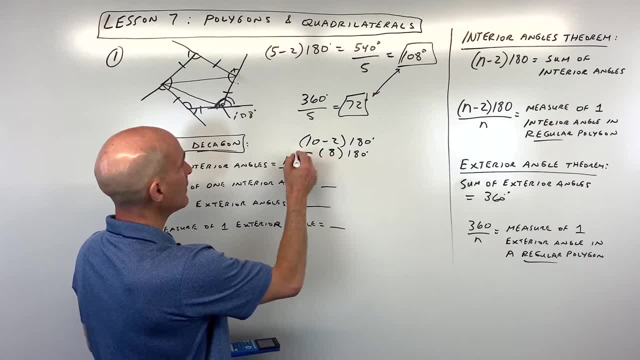 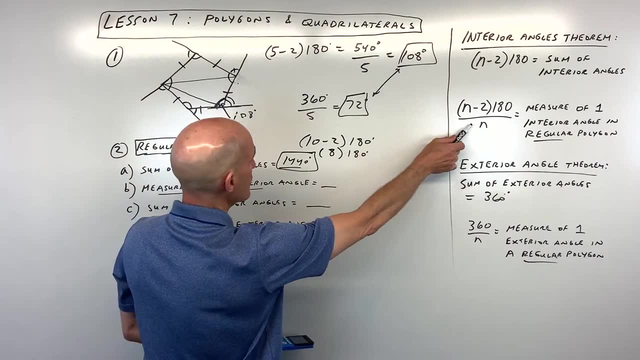 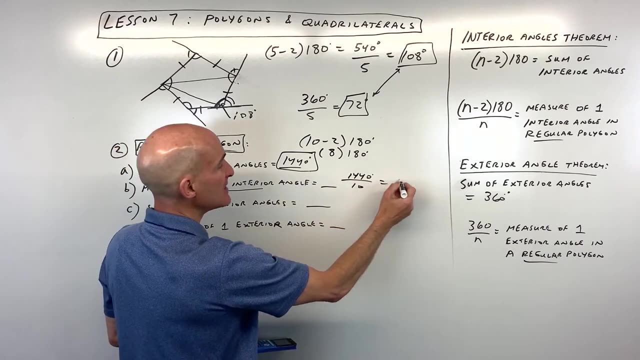 1,440.. So that's the sum of all those interior angles. Now, how much would the measure of just one interior angle be? Well, we can use this formula here. We could say: there's 10,, right? So if we divide the total by 10, that means each. 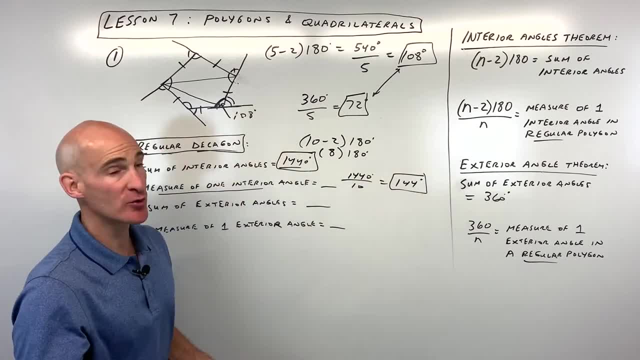 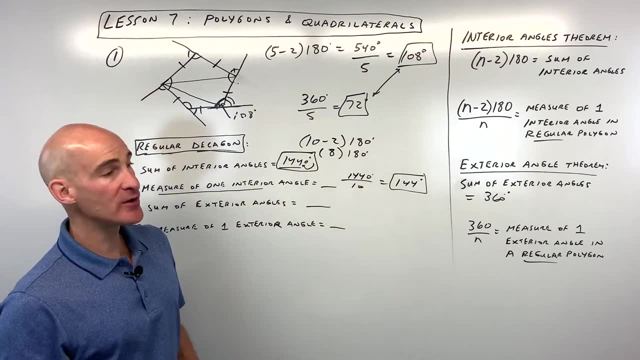 interior angle is going to be just 144 degrees. Of course, when you divide by 10, you just move that decimal one place to the left, And then the sum of exterior angles, all the exterior angles- are always going to add up to 360 degrees. So this is always going to be 360, regardless of the 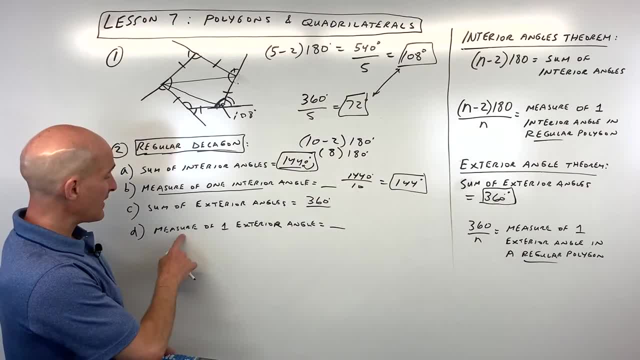 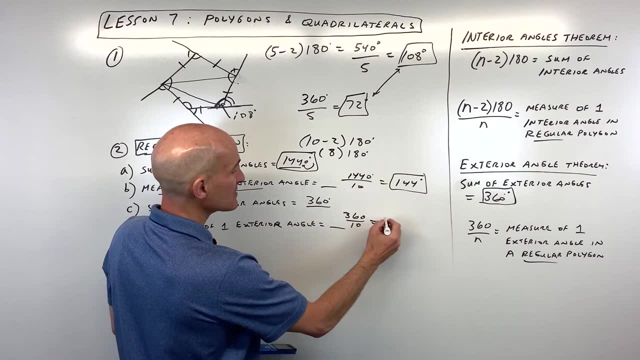 figure, whether it's a pentagon, hexagon, decagon, right, But then the measure of just one exterior angle. well, we could take 360 and divide it by 10.. Since there's 10 of them, that would be 36 degrees. 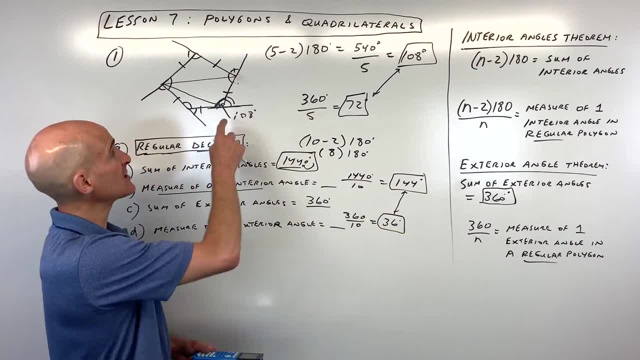 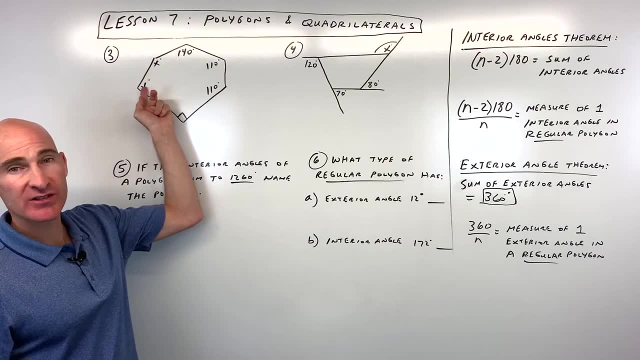 take 180 minus 144 to get 36.. Because remember how we said that they're a linear pair. Okay, so for number three. now, how would we find these missing angles? Well, what do you think? Well, we can see. these are, excuse me, interior angles, And we know all the interior angles. add: 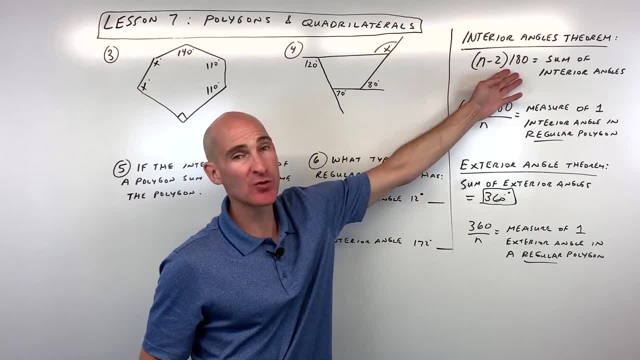 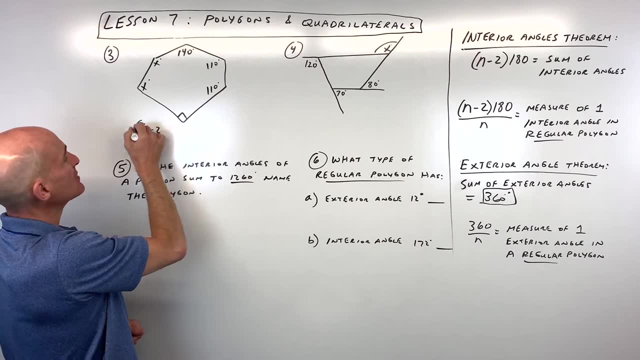 up to how much. Well, we can use this formula here: n minus 2 times 180.. But let's see how many angles we have: One, two, three, four, five, six. So we're looking at here is 6 minus 2, which is 4,. 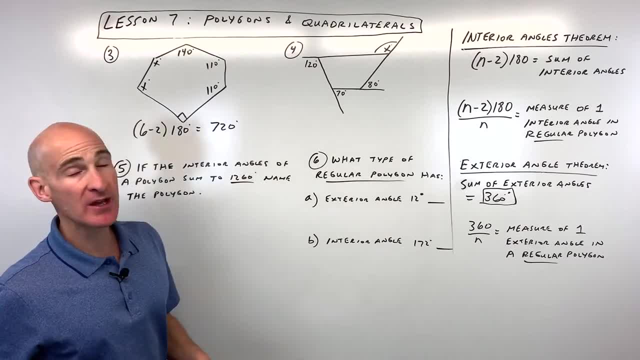 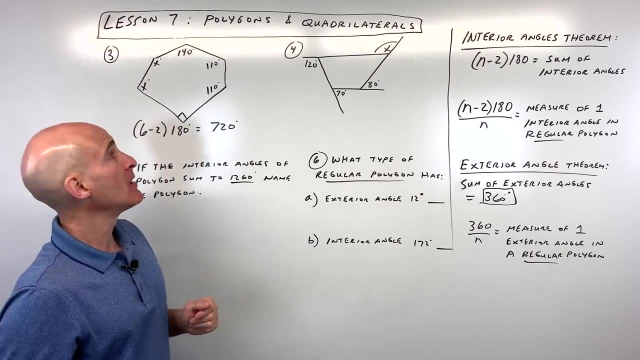 180, which is equal to 720 degrees. So if we make an equation and equal it to 100,- I'm sorry, 720 degrees, we can find that missing angle. These are the same, So let's go ahead and do that, So x. 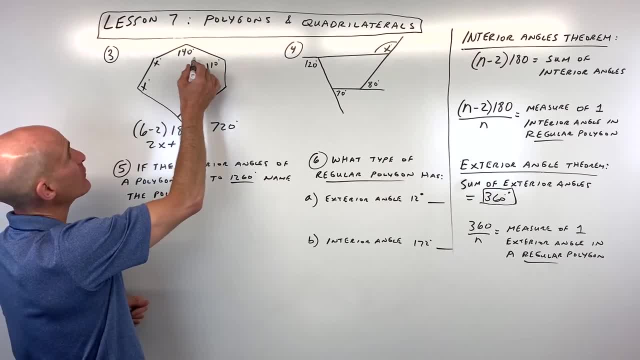 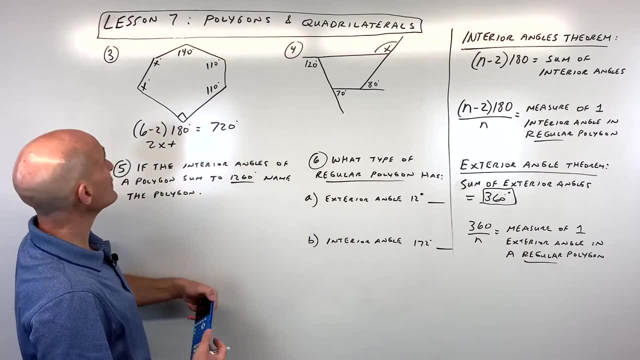 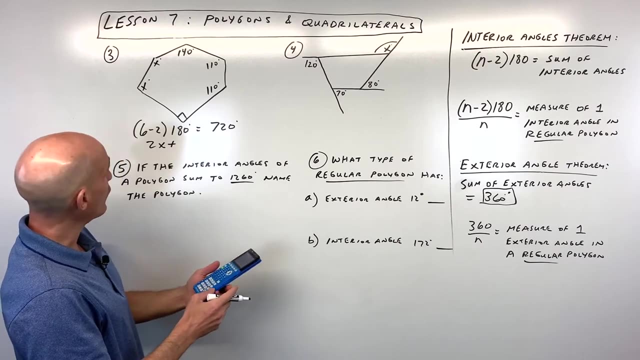 plus x is 2x plus 140 plus 110 plus 110 plus 90 equals 720.. Now let me go ahead and add up those angles. So this would be 220, 360 plus 90 would be how much 450.. So this is 450 equals 720. 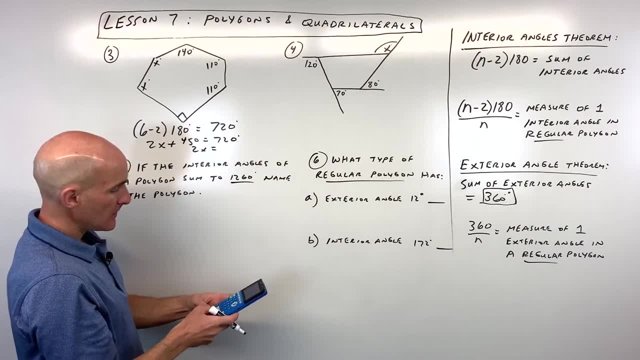 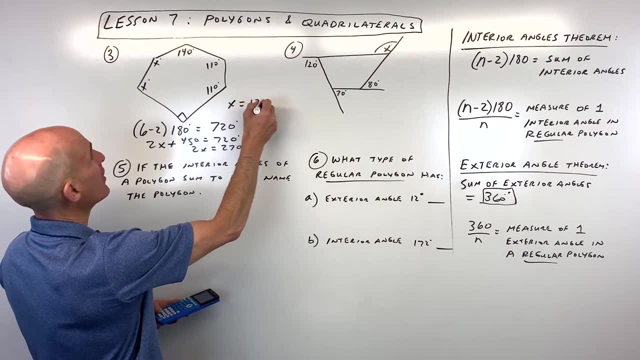 Subtract 450 from both sides and that gives us 270.. If we divide both sides by 2, you can see that x is equal to 135 degrees. and you got it. Okay, let's try number four now. What do you think? 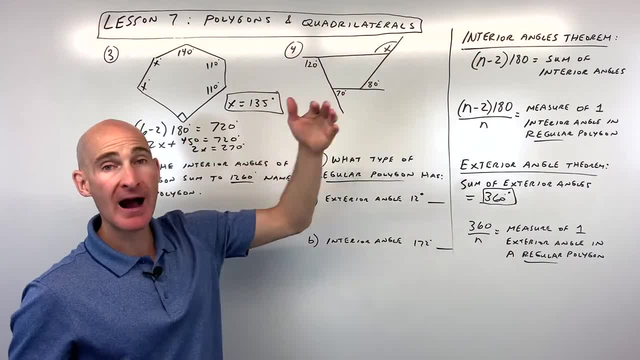 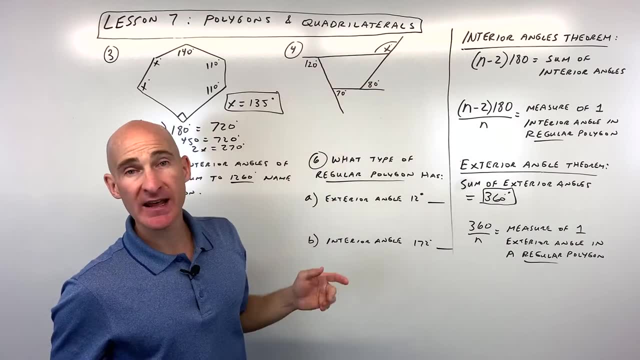 for this one. You can see these angles here are on the outside of the polygon. In this case it's a quadrilateral. You can see there's four sides, But the exterior angles, remember they always add up to how much 360 degrees. So what we can do is we can again make an equation. We can say 120. 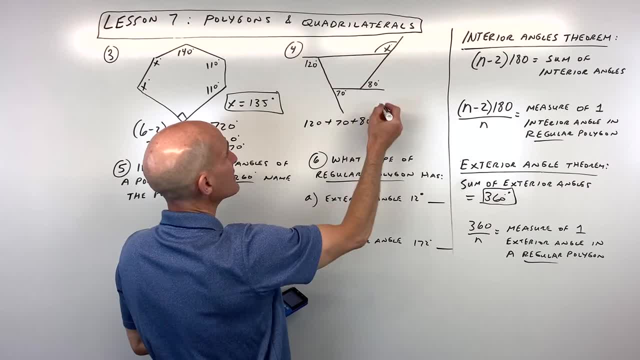 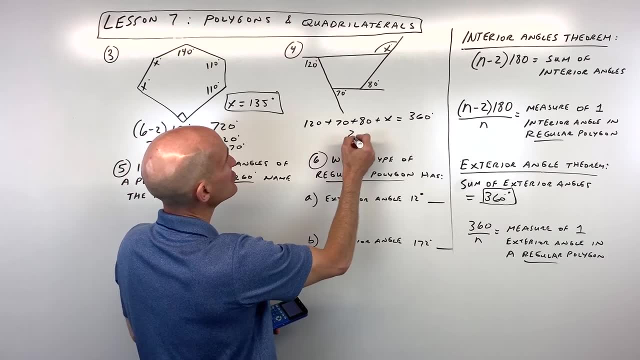 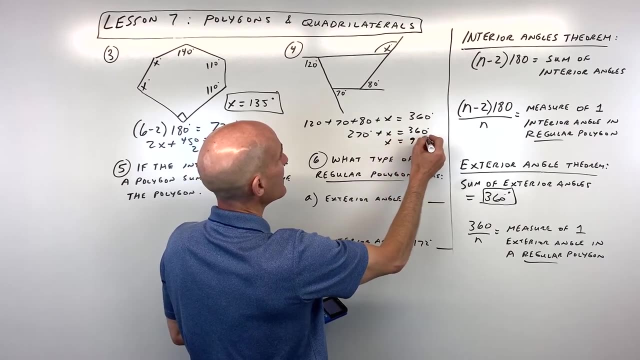 plus 70 plus 80 plus x equals 360.. So let's see This is 150 plus 120 is 270 plus x equals 360.. I'm sorry, subtract 270 from both sides and then that comes out to 90 degrees. Now you can see the. 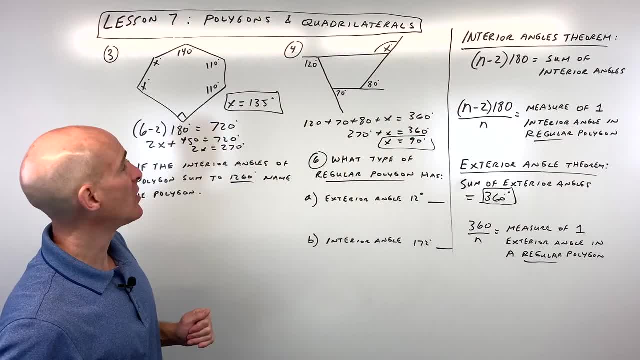 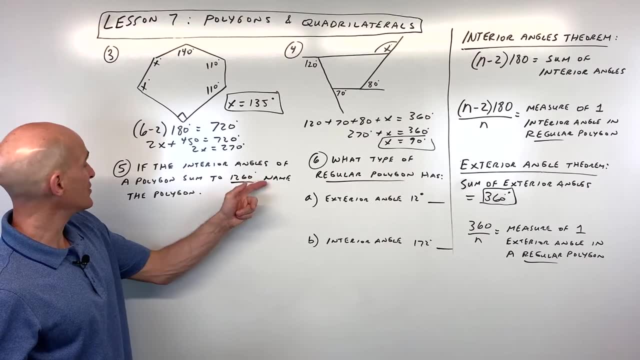 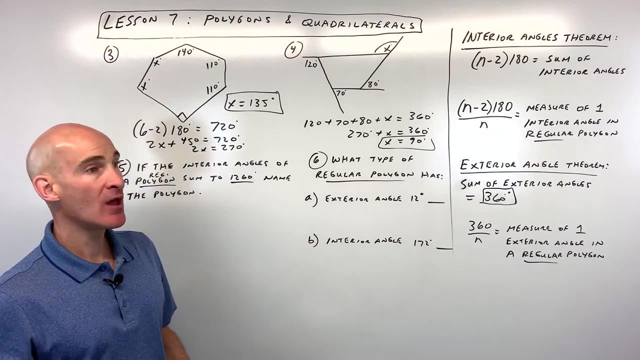 diagram is not drawn to scale. but again, that's how you would solve that one Number five. it says: if the interior angles of a polygon sum to 1,260,, name the polygon. And here what we're going to assume is that this is actually a regular polygon. So all the angles are the same, All the sides are. 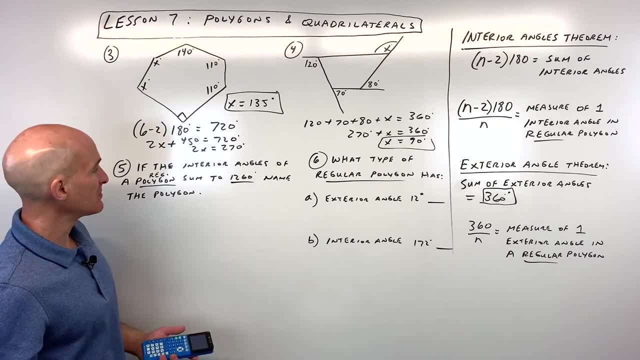 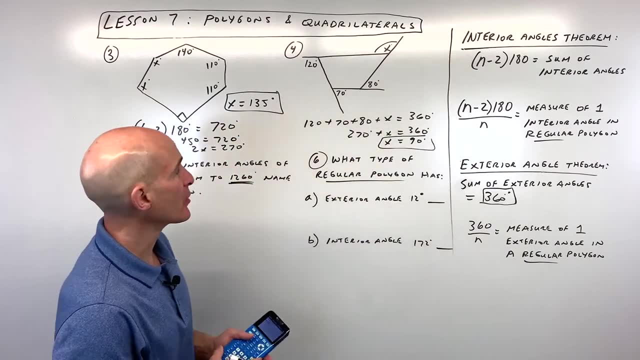 the same. In this case. it doesn't matter, It could be a regular polygon. It doesn't have to be a regular polygon, But if they all add up to 1,260, let's see. We'll use our interior angles theorem. We've got. 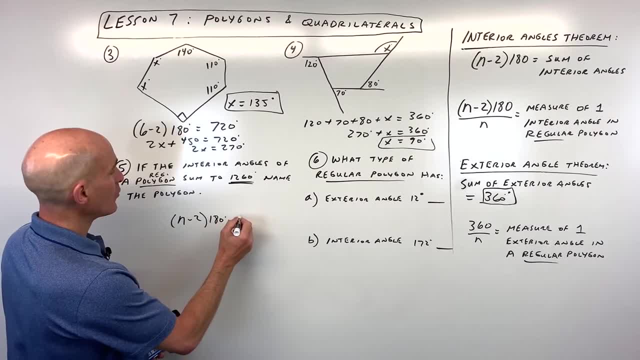 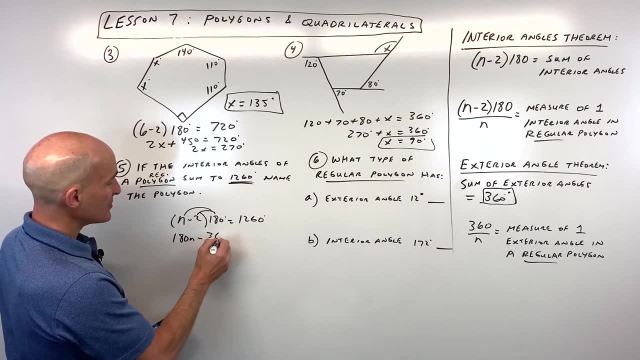 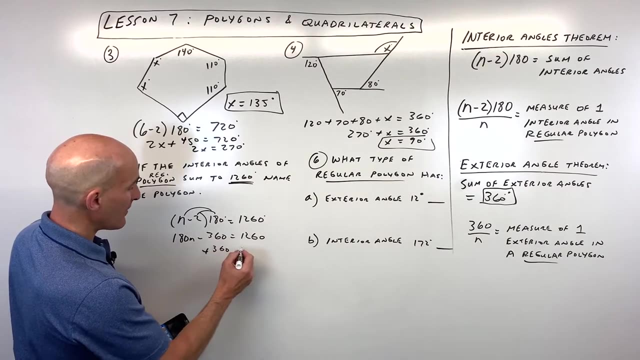 n minus 2 times 180 equals 1,260.. You can distribute the 180.. So that's going to give you 180n minus 360 equals 1260.. Let's see: Add 360 to both sides, Trying to get the variable n by 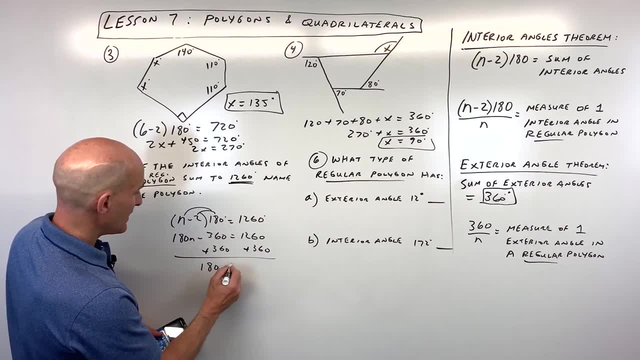 itself. So that comes out to 180n. equals, let's see 1260.. Plus the 360 is 1620.. And if we divide both sides by 180, let's see what that comes out to Nine. So 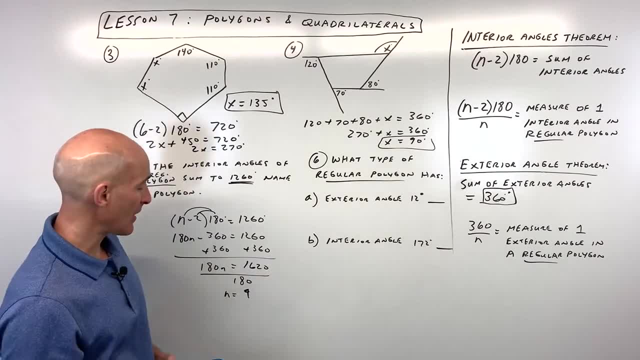 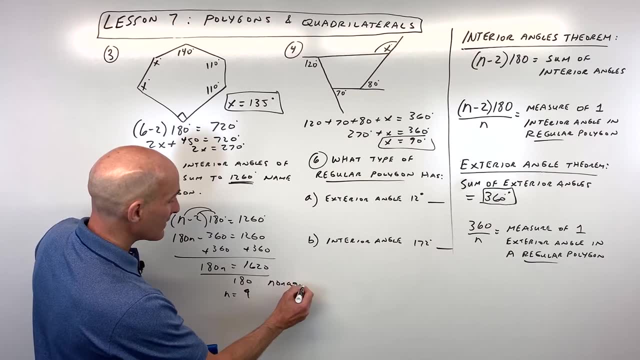 do you know what a nine-sided figure is? or an angle with a polygon with nine angles? Well, you could say it's a nine-gon, but we call it actually a non-agon. Kind of sounds like nine, doesn't it? 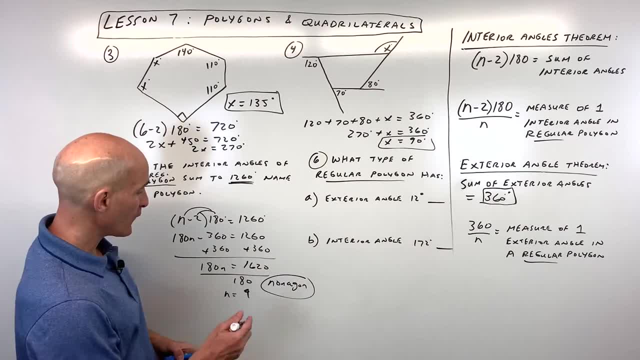 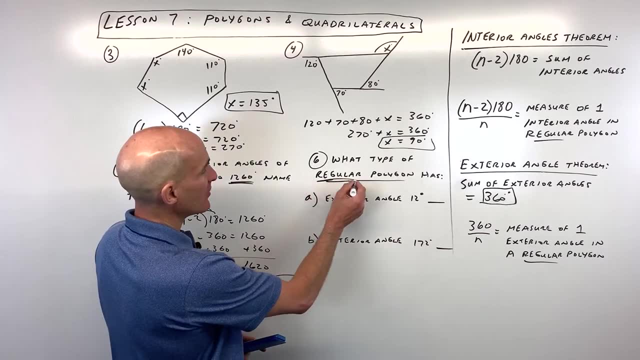 Non-agon, But if it's higher like 14, you can just say like 14-G-O-N, 14-gon. Okay for number six. now it says what type of regular polygon- okay, here's a regular one- has an exterior angle. 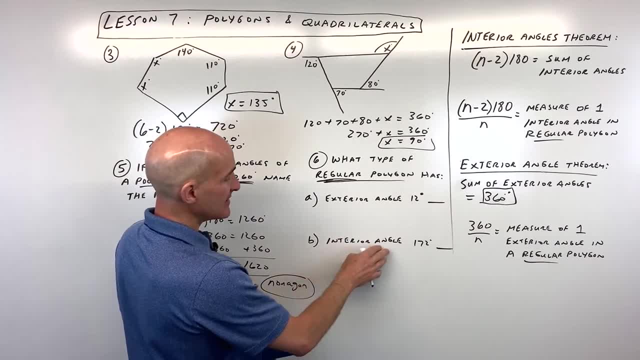 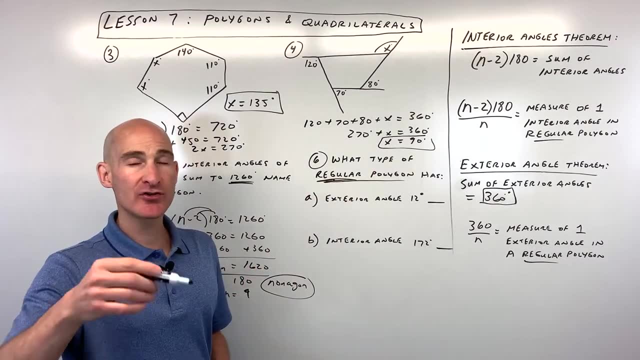 of 12 degrees, And then this is a separate problem. It has an interior angle of 172 degrees. Let's do the exterior angle one first. Well, if it's a regular polygon, all those exterior angles are the same. We can use this formula right here to find the measure of one of the exterior angles. 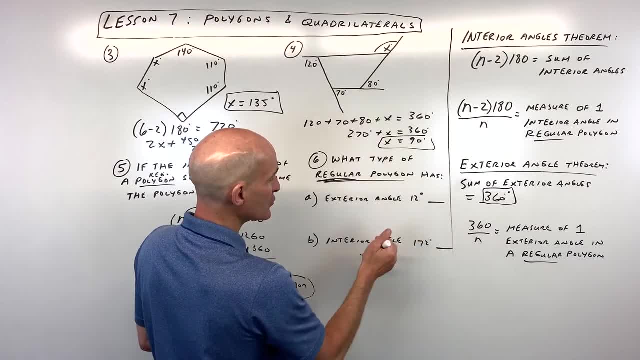 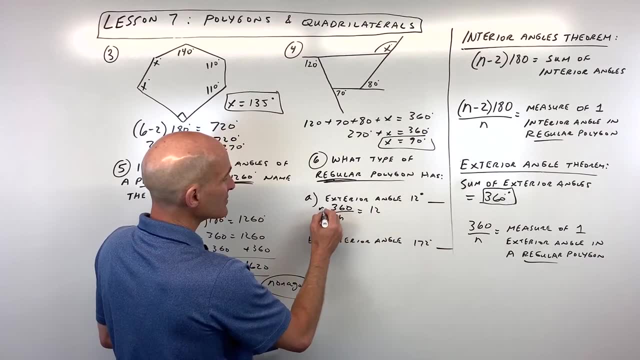 They all add up to 360.. If we divide by how many there are, we'll get the measure of just one, So let's go ahead and do that. So 360 divided by n equals 12.. I could multiply both sides by n to get rid of this fraction here. So we have 12n equals 360.. 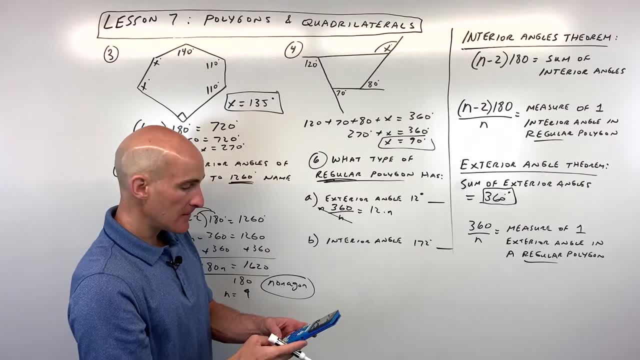 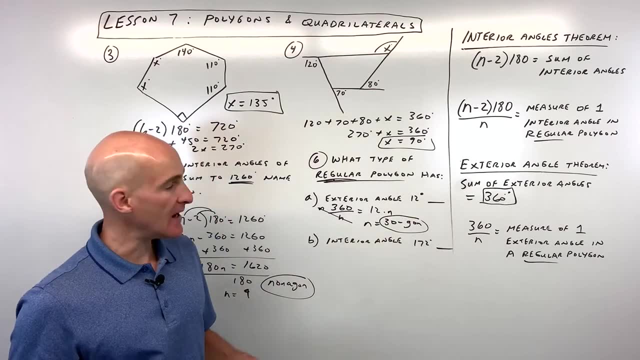 And if we divide both sides by 12, we get 30. So this is a 30-gon Okay. I mean he has 30 angles or 30 sides, And then this one, an interior angle of 172 degrees. Now again remember. 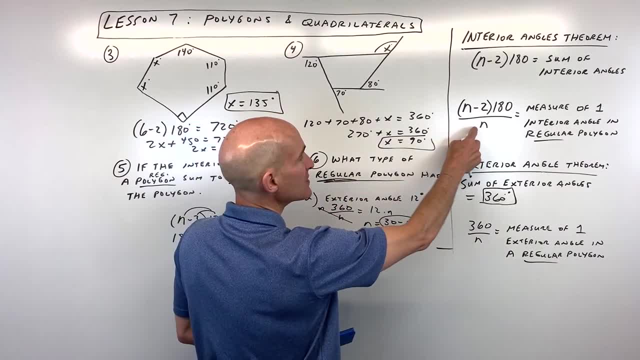 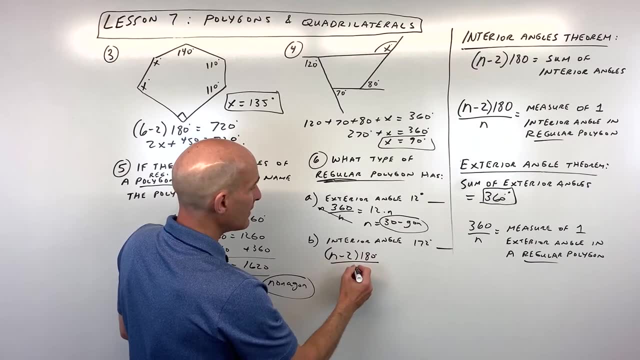 this is a regular polygon. If we want to find the measure of just one of the interior angles, we can use this formula right here, And we can say n minus two times 180.. Divided by n equals 172 degrees for our interior angle If we multiply both sides by n. 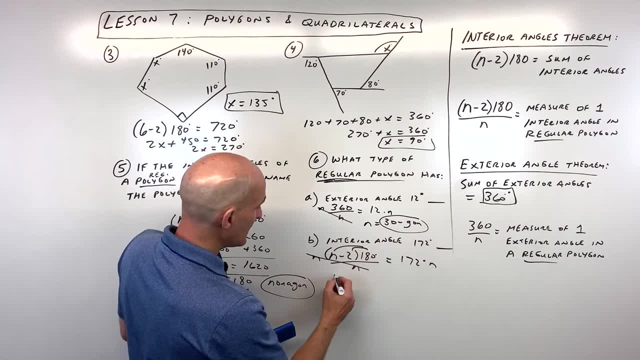 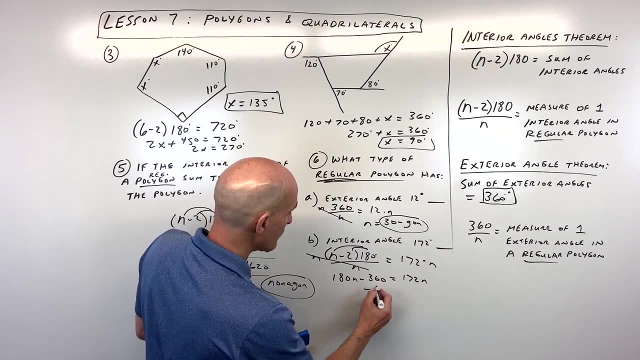 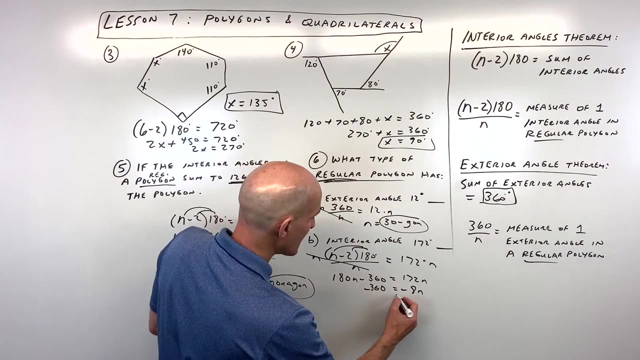 say left and right. to keep that balanced, we can distribute the 180. We get 180n minus 360 equals 172n. If we subtract 180 from both sides that comes out to a negative 8n. And if we divide both sides by negative 8, what does that come out to? 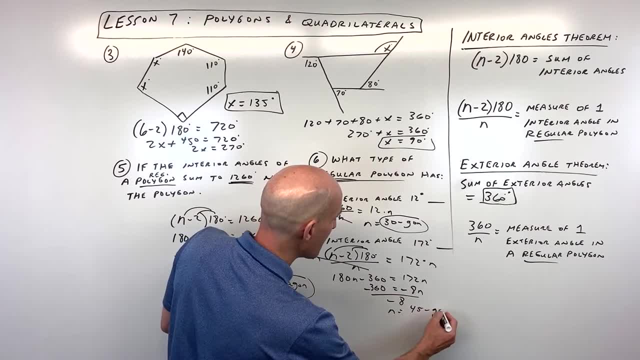 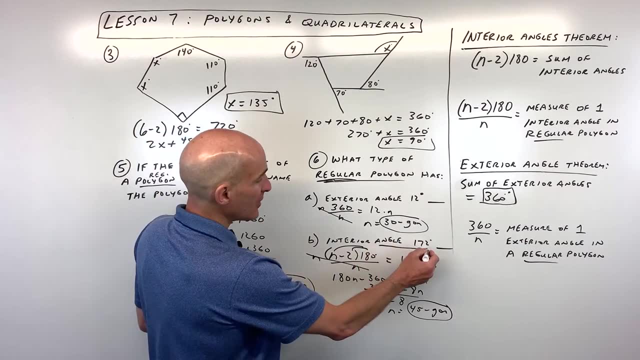 45. So this is actually a 45-gon, meaning it has 45 sides or 45 angles. Now you might have said, Mario, we know that. you know, if the interior angle is 172, that means the exterior angle is. 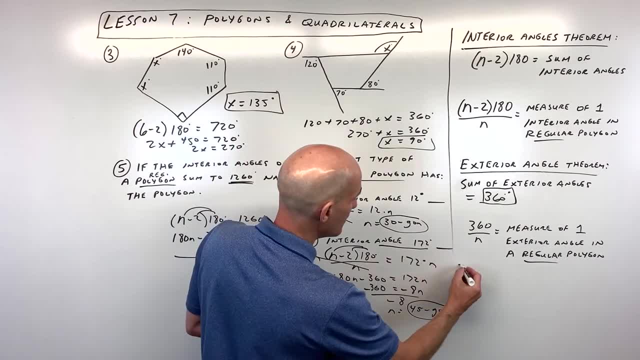 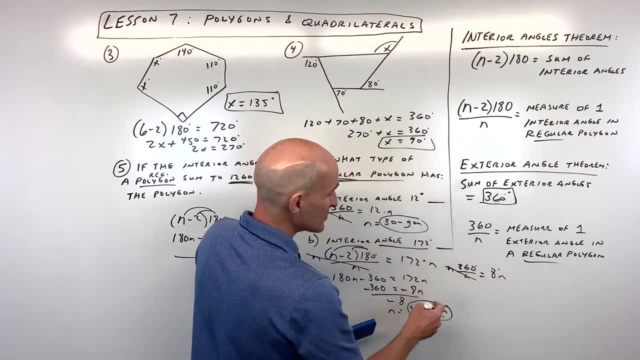 8, because they have to add up to 180.. So we could have used this formula right here: 360 divided by n equals 8 degrees. Multiply both sides by n, and then you could say 360 divided by 8, and you're going to get again a 45-gon. So sometimes it's easier to use this formula. 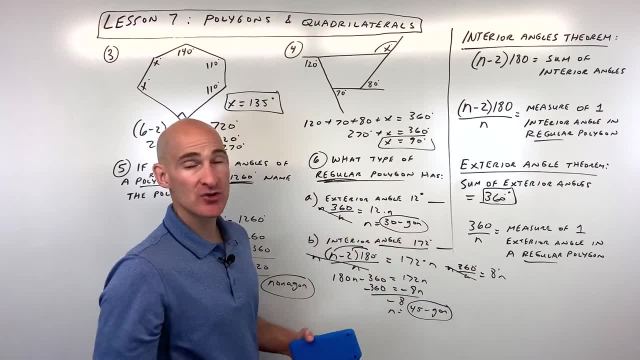 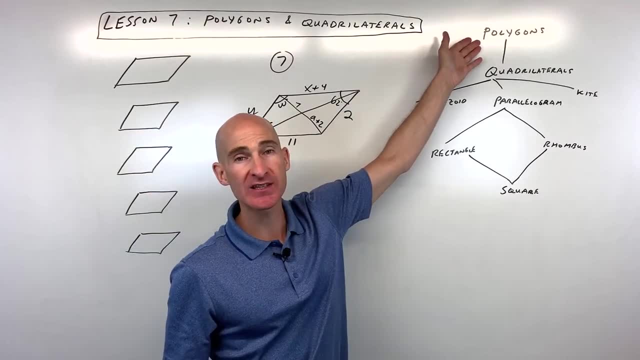 because it's a little bit simpler, a little bit easier to work. just remember that those two angles are supplementary. Okay, now we're going to switch gears a little bit. We've been talking about polygons in a general sense. Now we're. 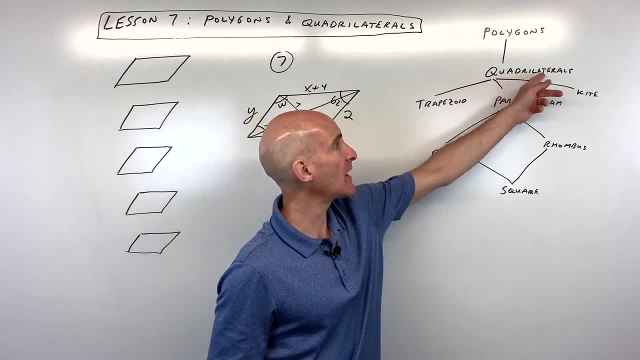 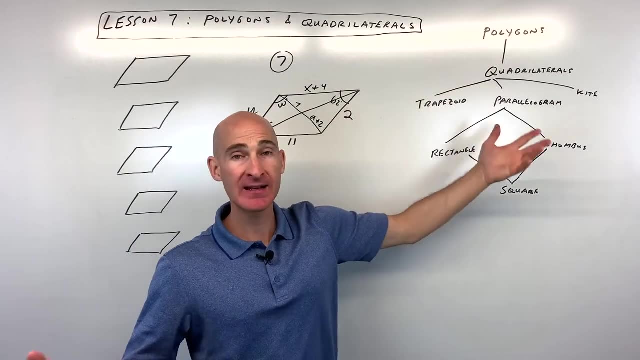 going to switch to a particular type of polygon which is a quadrilateral. Remember, quad means four, lateral means side. So this is a four-sided figure that we're working with, as opposed to just like any type of polygon, like a pentagon or a decagon. But you can see with this tree diagram. 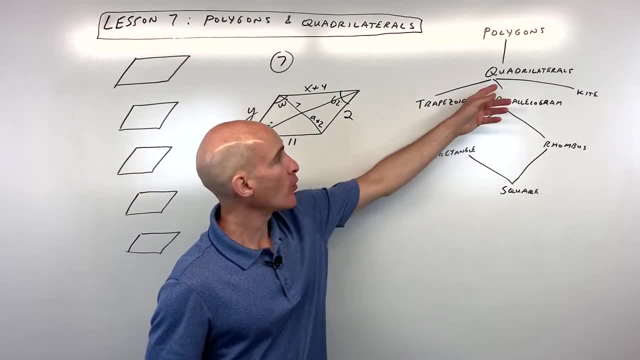 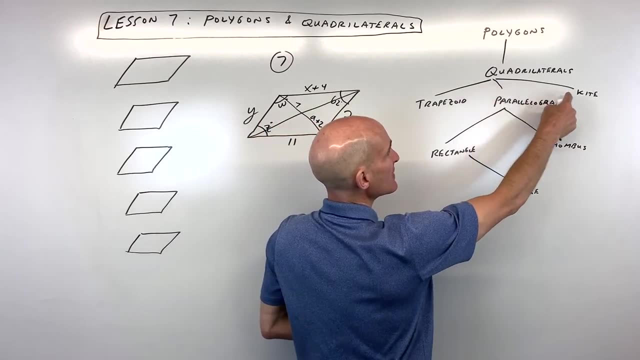 here I've tried to illustrate where we're going in this lesson. So quadrilaterals are polygons of four sides, but then we're going to be looking at trapezoids, parallelograms and kites, which are all types of quadrilaterals And then parallelograms. we're going to then look at some. 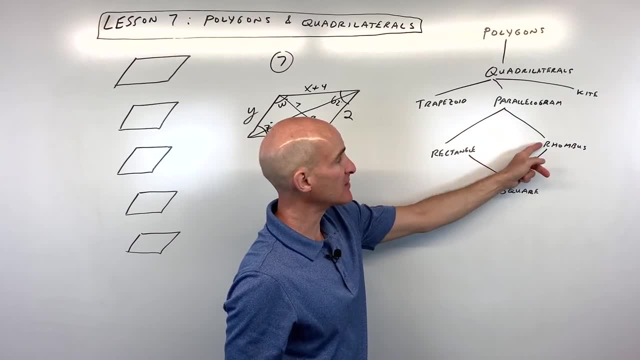 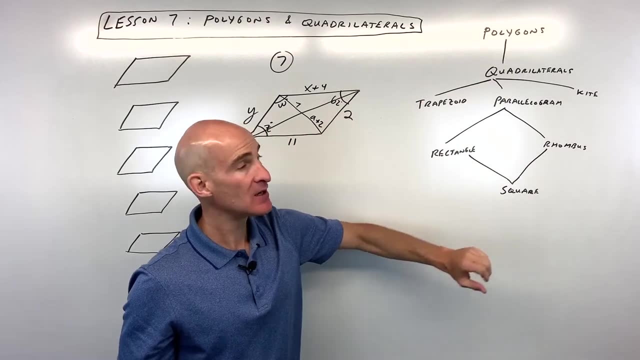 particular types of parallelograms, like rectangles, rhombus and square. Okay, notice: a square is a combination of a rectangle and a rhombus, So you might want to memorize this diagram or put it in your notes to see how all these figures are related. We're going to be going through each 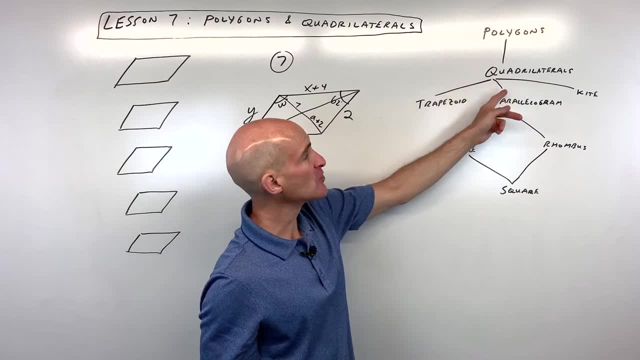 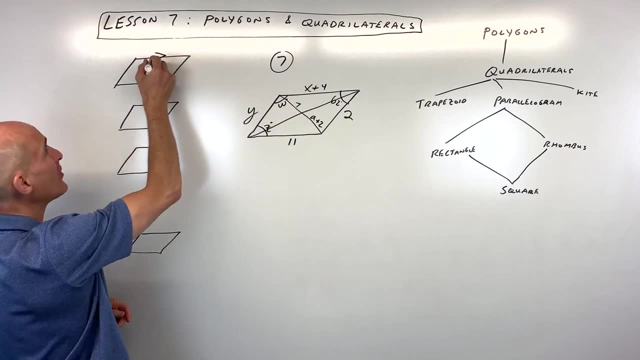 of the different types, But starting off with quadrilaterals, but more specifically, parallelograms, what exactly is a parallelogram? Well, a parallelogram, just like it sounds. the opposite sides are parallel And that's what these little arrows represent, that these two 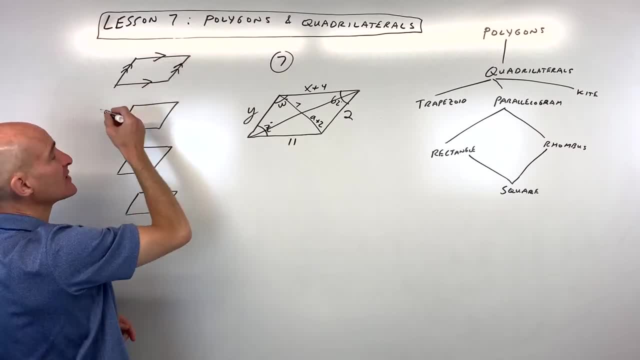 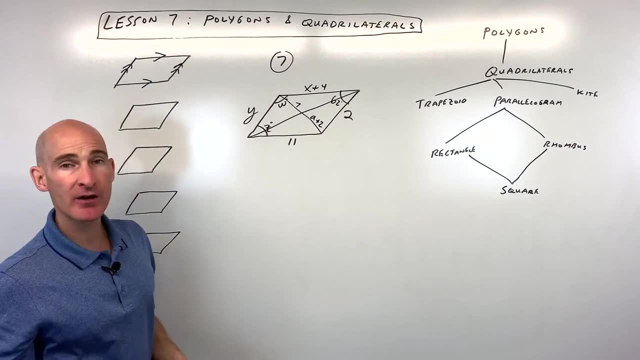 sides are parallel. If they were to keep going, they wouldn't cross. These two sides are parallel. If they kept going, they wouldn't cross, And that's our parallelogram. But what we're going to do now is we're going to talk about all the different properties of parallelograms. You're going to 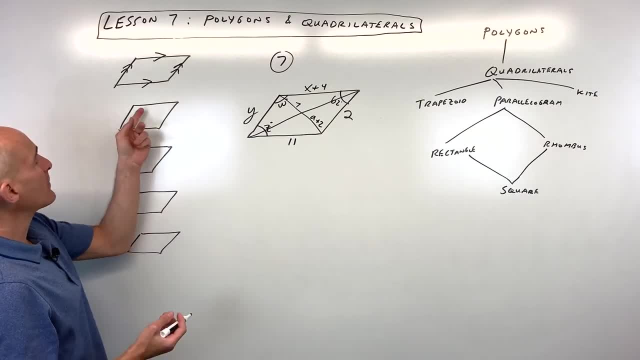 want to memorize these, And so let's go ahead and do that. So in a parallelogram, if we know it's parallel, we automatically know that both pairs of opposite sides are congruent, meaning they're the same length. We also know that both pairs of opposite angles are congruent, So these are equal. 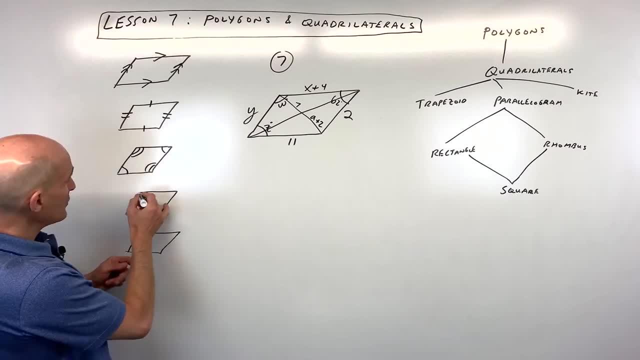 and these ones across from each other are equal. And we also know that the diagonals, okay these ones that connect the opposite vertices, they bisect one another. What that means bisect? bi means two, sect means cut. So what they're doing is they're cutting each other in half. So, for example, 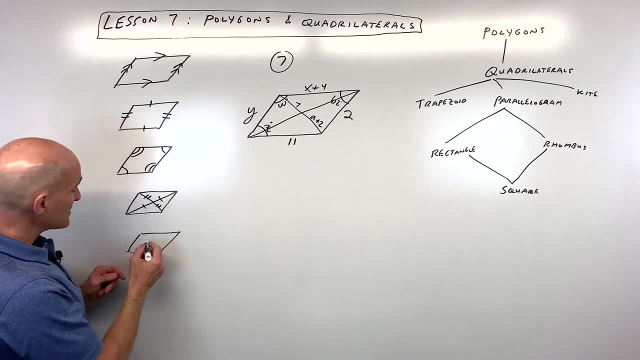 if I'm going to cut and they're cutting one another, then they're creating a diagonal and then they're cutting one another and then they're cutting one another. So these are the two, two additional segments that they're going to add up to 80. And these two segments are going to be: 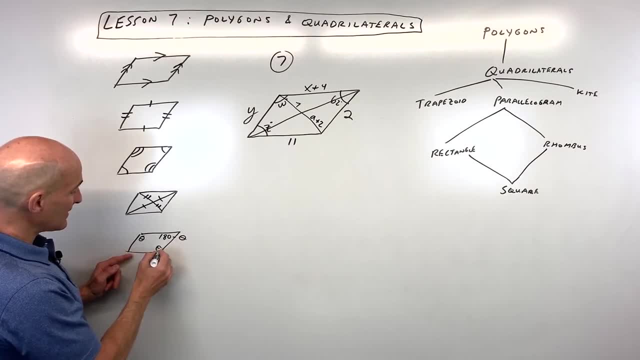 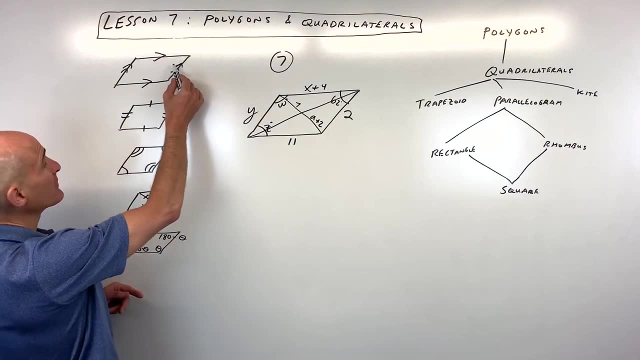 congruent. And then the last one is that if you look at the consecutive angles- so for example, if this was like theta or x- this angle that's like next to it is going to be 180 minus theta. These ones across from each other are the same. that's theta. This one over here is going to be 180 minus theta. So what I mean by that is 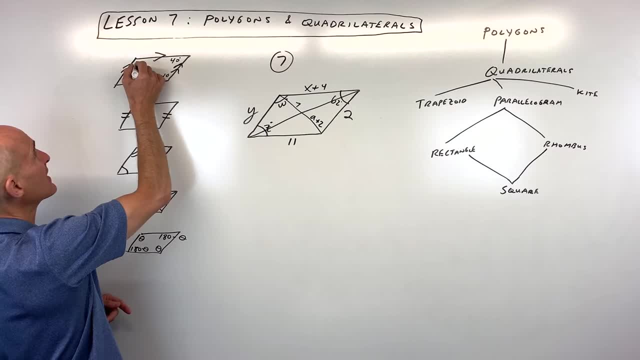 140 plus 40 is 180.. This one plus this one has to add up to 180.. So that's 140.. Of course, the ones that are across from each other are congruent, And the reason this works is we talked about in an 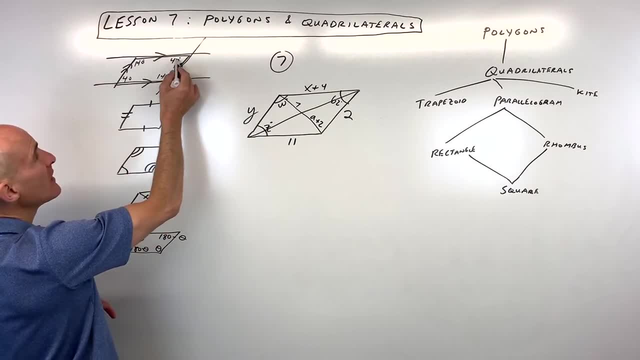 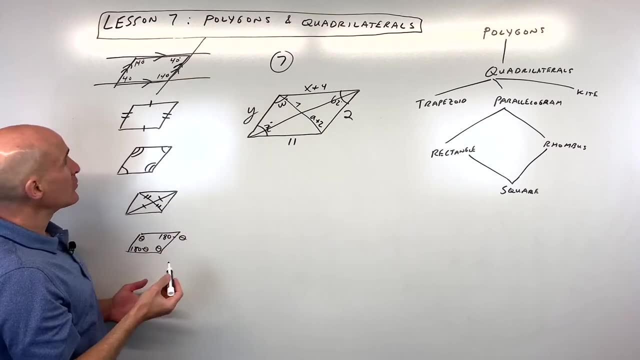 earlier lesson, parallel lines cut by a transversal. These are what are called consecutive interior angles or same side interior angles, and those are always supplementary. So you know, this all comes from the parallel lines and congruent triangles we talked about in earlier lessons. But you want 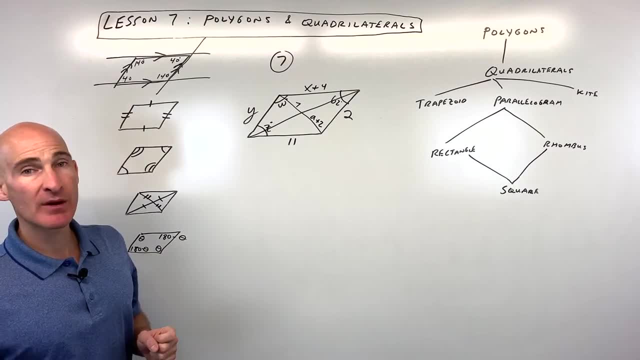 to memorize these properties so that you can apply them to some of these upcoming problems. For number seven, let's go ahead and solve for these missing quantities here, these missing variables. So first thing I notice is this is a parallelogram. Okay, that's given, But you can see. 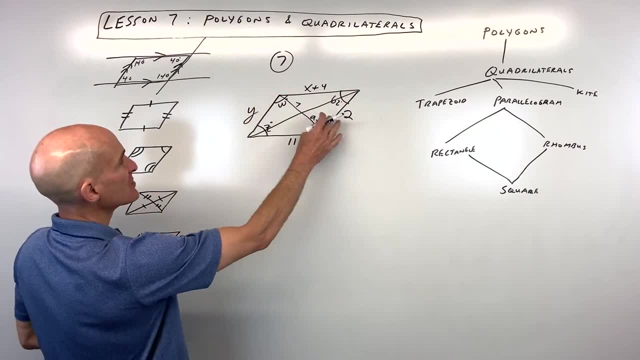 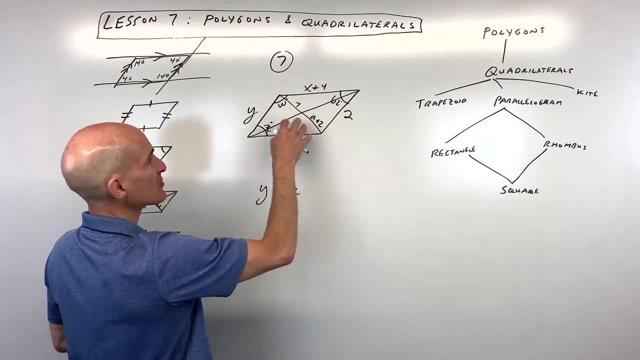 that the opposite sides are going to be congruent. So that means if this is two, that means that y is also going to be two. If this is x plus four, this is eleven. The opposite sides are congruent, So x plus four equals eleven. We can solve that equation. That means x is going to equal seven. 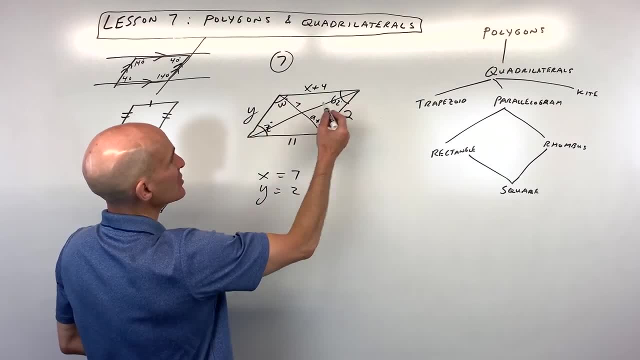 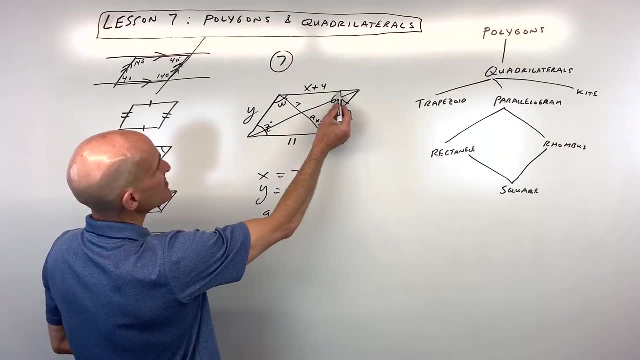 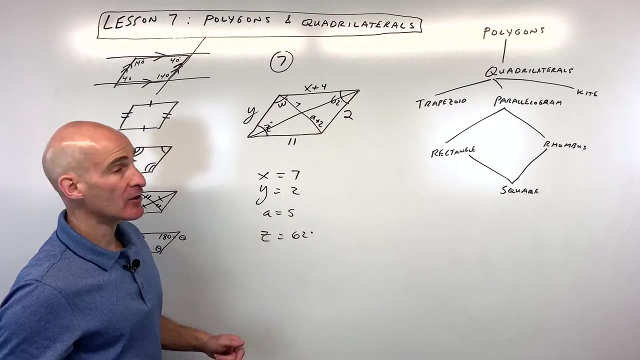 Here you can see that the diagonals, they bisect each other. So that means that a plus two has to equal seven. So that means a must equal five. We have this is 62 degrees. So we know that angle z here must also be 62 degrees, Because the opposite angles are congruent. And then over here. 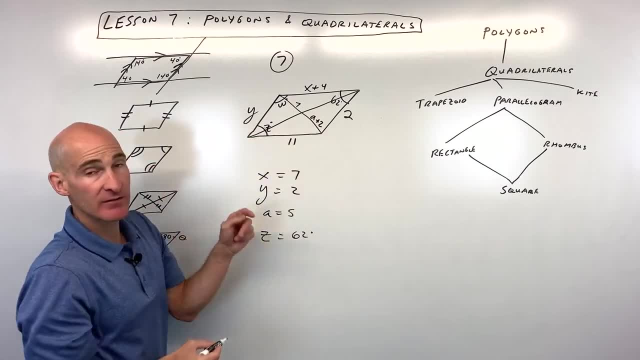 these two angles are consecutive angles And they're going to be supplementary. so if this is 62, we know that w is equal 180 degrees. From here we have z equals two And they're going to be supplementary. So if this is sixty-two, we know that w is equal 180 degrees. From here we have фильма. 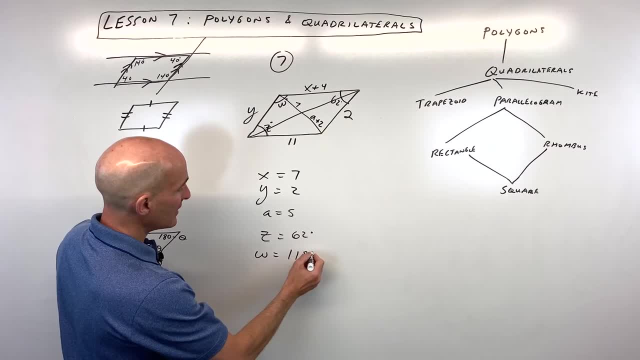 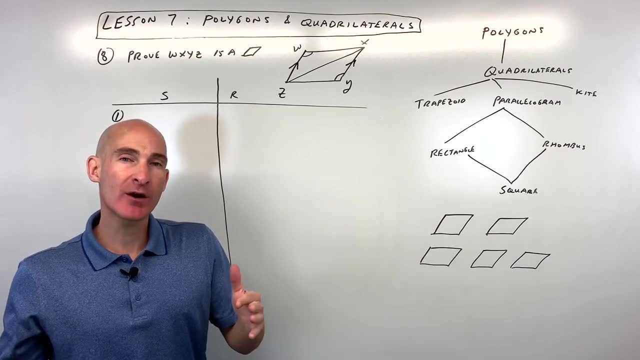 180 minus 62,, which is how much? 118 degrees, and you've got it. Okay, now we talked about the properties of parallelograms. Now we're gonna talk about how do you prove that a quadrilateral is a parallelogram, right? 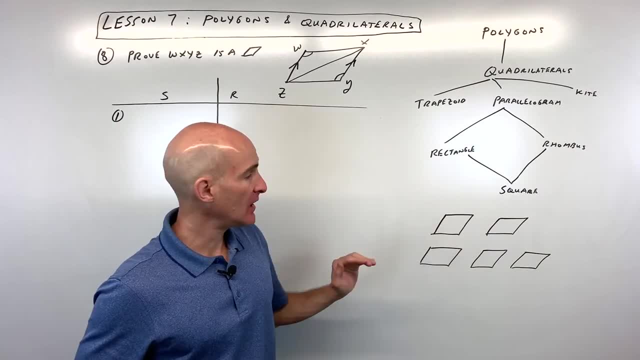 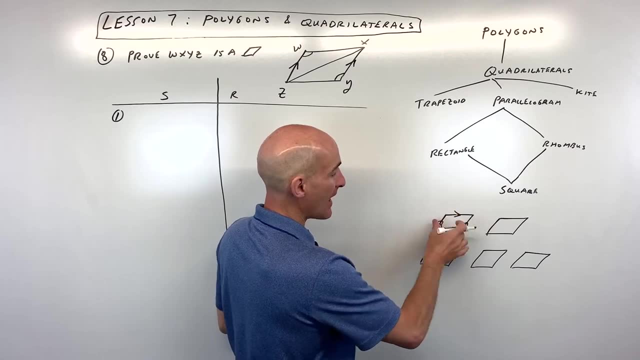 Well, let's talk about the five main ways, okay? One way to do it, of course, is to use the definition of a parallelogram and show that both pairs of opposite sides are parallel. Then you've proved it's a parallelogram. 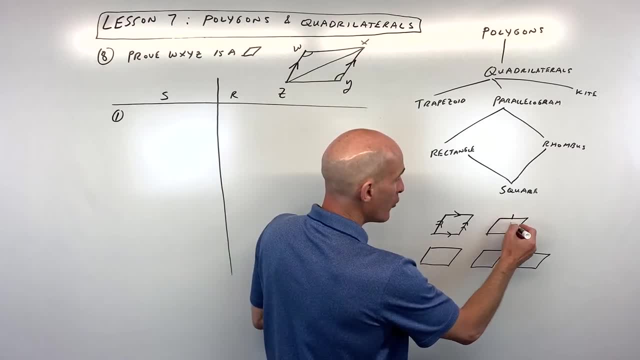 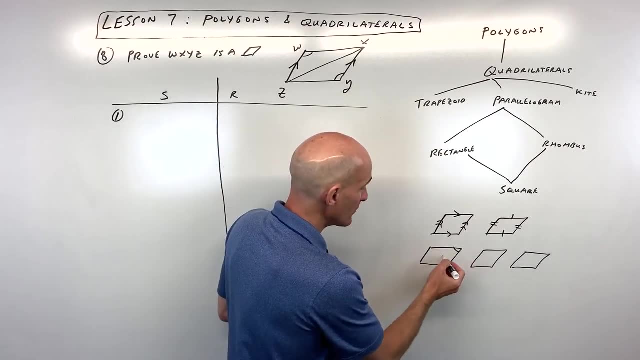 by definition right. Another way to do it is to show that both pairs of opposite sides are congruent. Then you've proved that it's a parallelogram. You could also show that both pairs of opposite angles are congruent. That proves that it's a parallelogram. 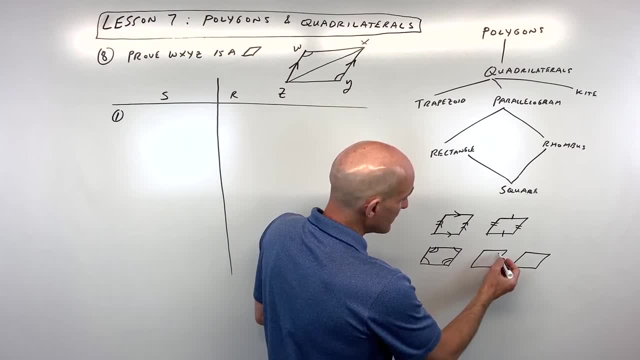 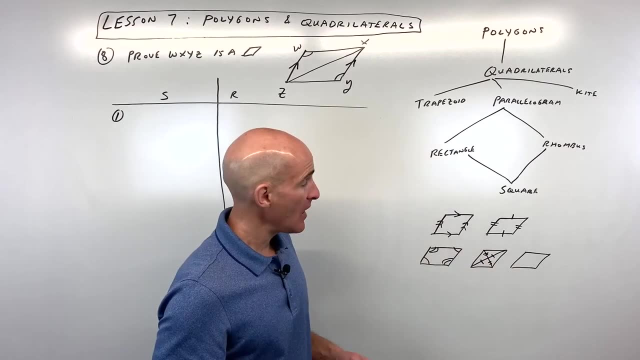 You can also show that. let's see the diagonals bisect each other, meaning they cut one another in half right. And the last one. this is the one that students oftentimes forget. I hope you don't forget this one. 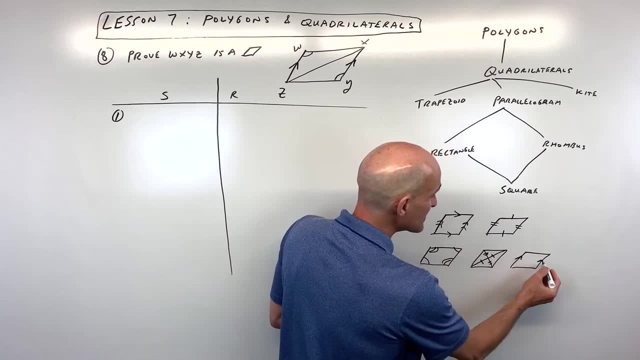 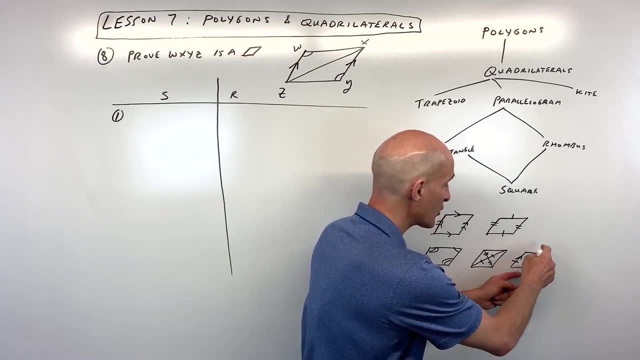 is you wanna show that one pair of opposite sides are parallel- that's what the arrows represent- and congruent, that's what the dashes represent. So it could either be these two sides are parallel and congruent, or the top and the bottom. 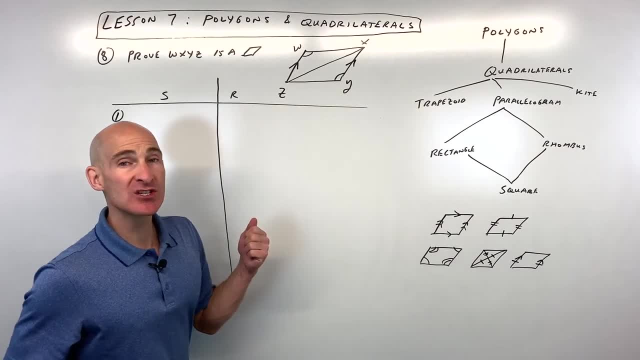 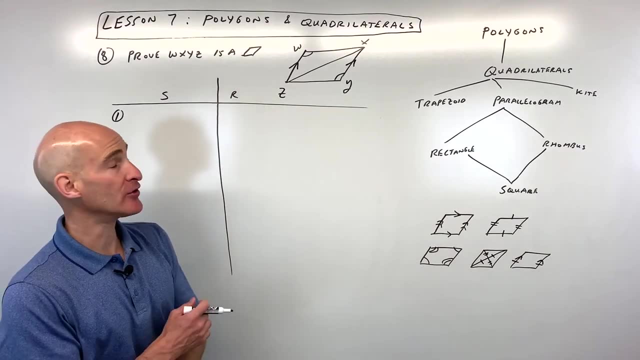 those two sides are parallel and congruent. So now what I wanna show you is just an example of how to prove that a quadrilateral's a parallelogram, in a two-column proof style, like you did with triangles. So here it says: prove that quadrilateral WXYZ. 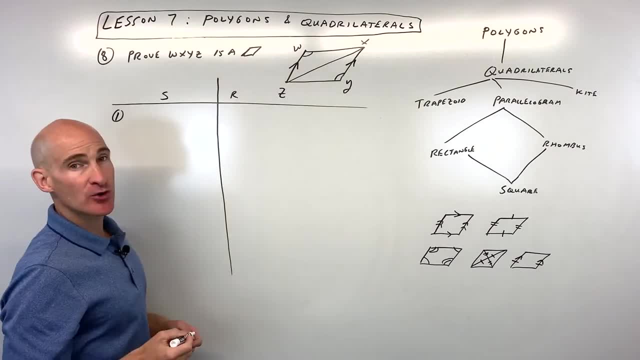 over. here is a parallelogram. This is just kind of the shorthand symbol for parallelogram And let's see. so it looks like they gave us an. angle W is congruent to angle Y, so let's write that down. 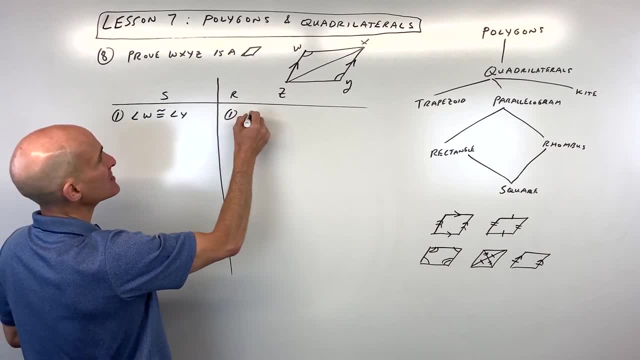 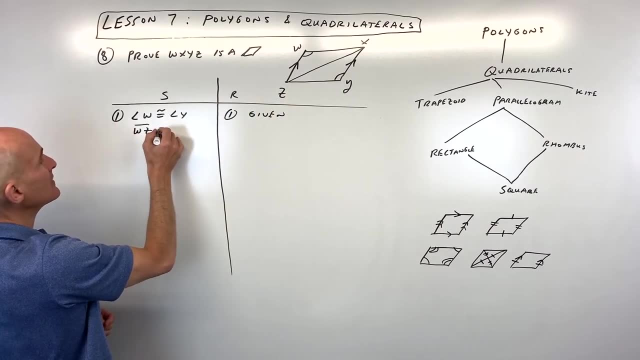 Angle W is congruent to angle Y. That, of course, is given from the diagram, And we also know that WZ, segment WZ, is parallel to segment XY, and that was also given. Okay, let's go to step number two now. 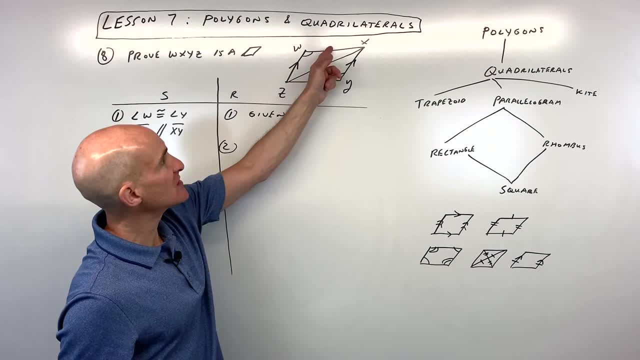 So we're trying to prove that this is a parallelogram. If we could show that these two sides were parallel- we already know these two sides are parallel- We could prove it's a parallelogram by definition of a parallelogram. 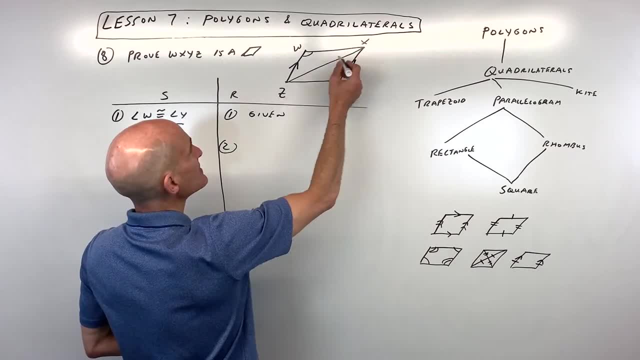 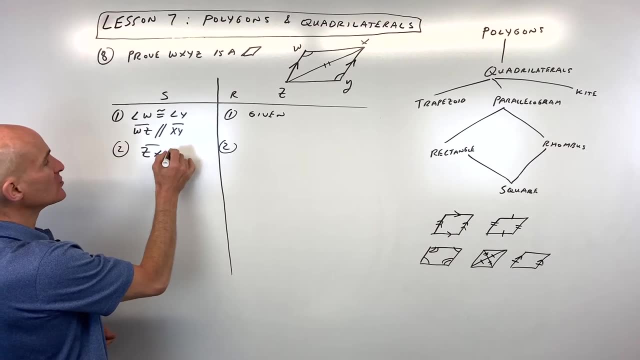 But let's see if there's another way we could do this. Well, we know that ZX is congruent to ZX because it's shear between these two triangles, right? So what's that called when anything is congruent to itself? Remember that from when we talked about triangles. 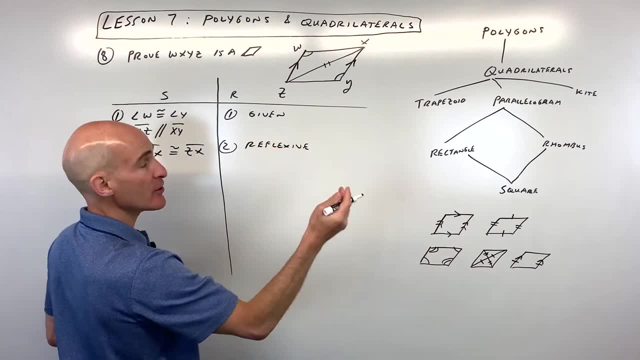 That's the reflexive property, Kind of like when you look at a mirror, your reflection- you're the same height of the mirror as you are in real life. Now notice that these are parallel lines. Sometimes when I have parallel lines, 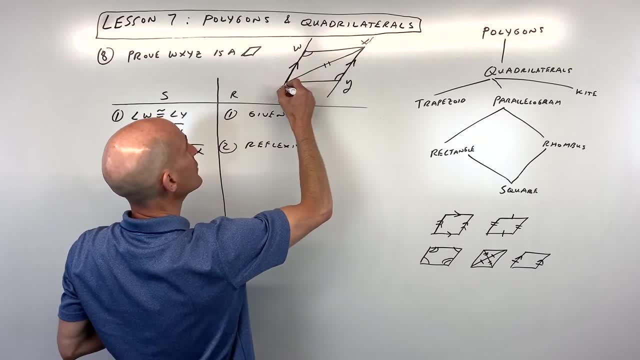 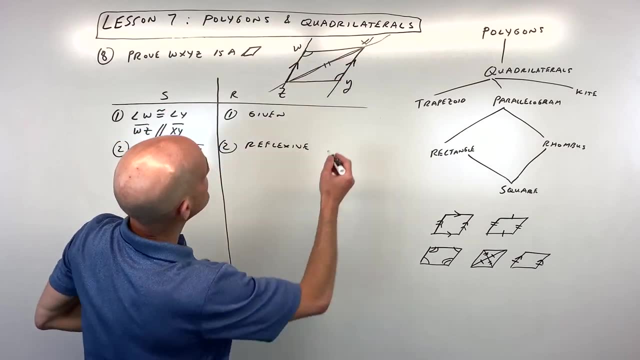 what I like to do is I like to kind of extend them a little bit, make them a little bit longer, And this transversal you can extend a little bit longer. If you take this and you rotate it, what you'll notice is that this angle here 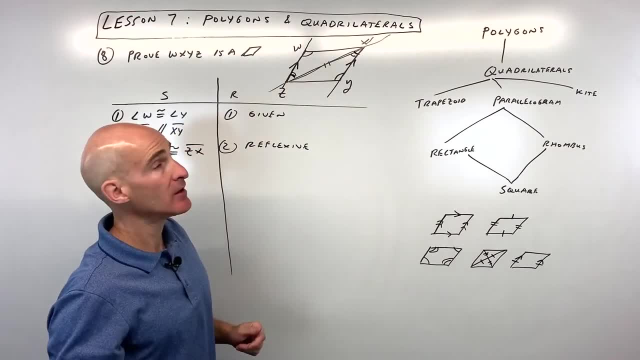 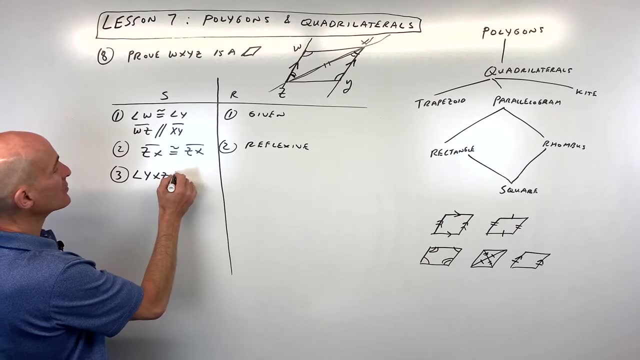 and this angle here are congruent. okay, And why would that be? See, if you can figure that out, Let me write down the angles. This is: angle YXZ is congruent to angle WZX, So why are those congruent? 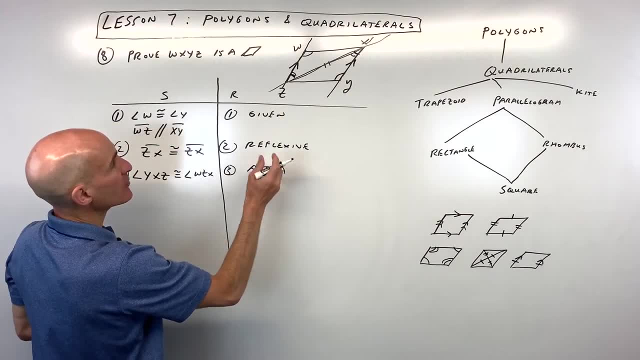 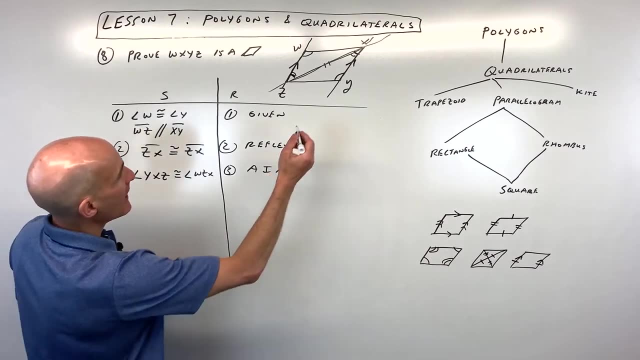 Alternate interior angles. One's on the left, one's on the right. They're in between the two parallel lines, you know, on either side of that transversal alternate interior angles. So now look at what we have. We've got this triangle and this triangle. 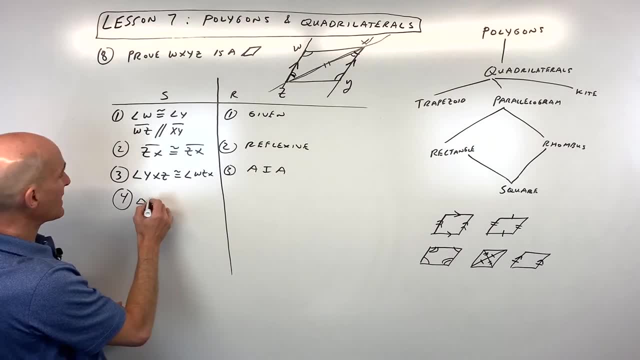 Why do you think those two triangles are congruent? So why would triangle YXZ be congruent to this entire triangle WZX? Hmm, why do you think for that? Well, you can see that's angle, angle side right. 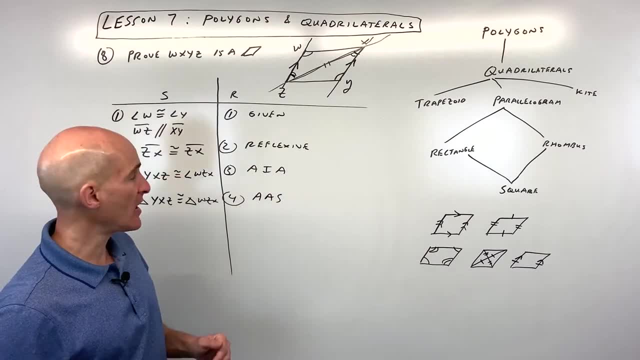 So you've got angle angle side. You want to make sure you go in order as you go around the triangles: Angle the next angle, you come to the next side. So now we know the triangles are congruent. Why is that useful to us? 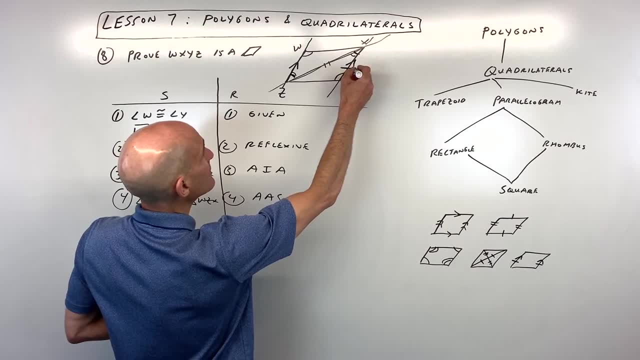 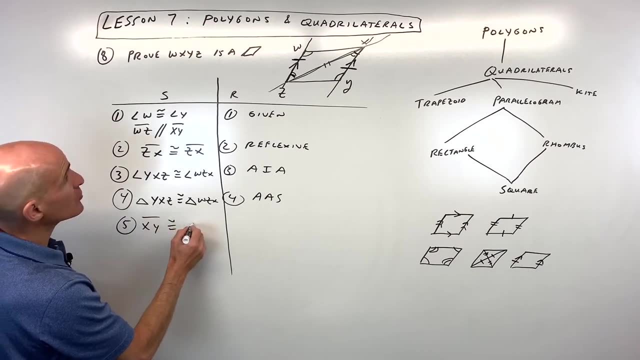 Well then I could say that this side is congruent to this side. Let's write that down. And why is that true? Segment XY is congruent to segment ZW. we'll just say Okay, or you can say WZ, either order. 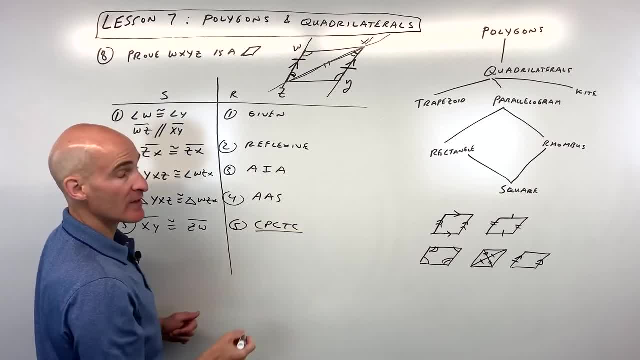 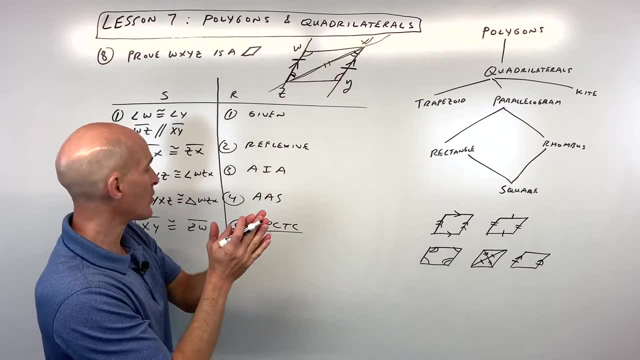 That's going to be because of the CPCTC. Remember that acronym. corresponding parts of congruent triangles are congruent, meaning the parts that match up. Once we prove these triangles congruent, the parts that match up are also going to be congruent. 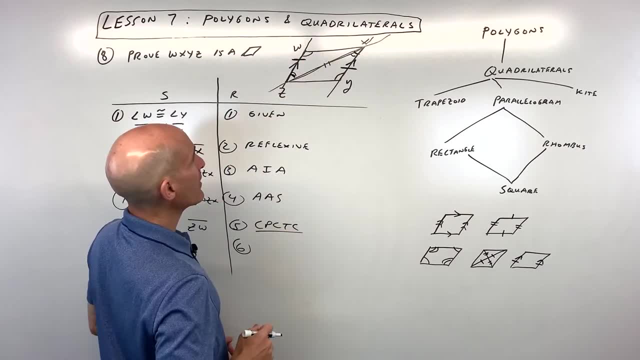 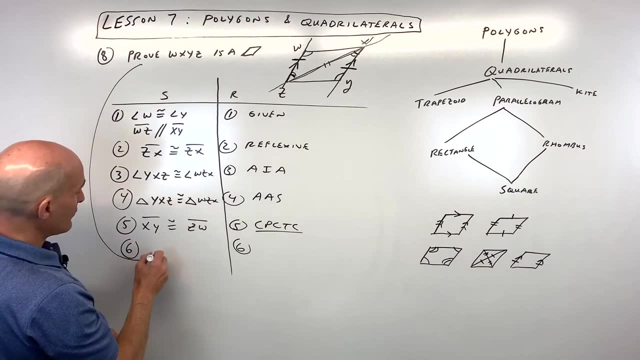 And then the last step: why are these? why is this? quadrilateral, a parallelogram? Hmm, what do you think for that? So I'm going to say it is a parallelogram, right, And the reason is because you have one pair. 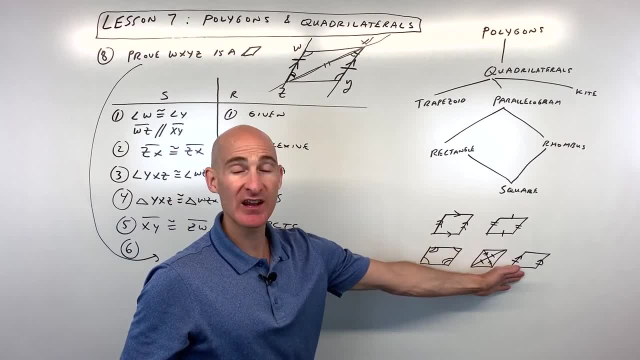 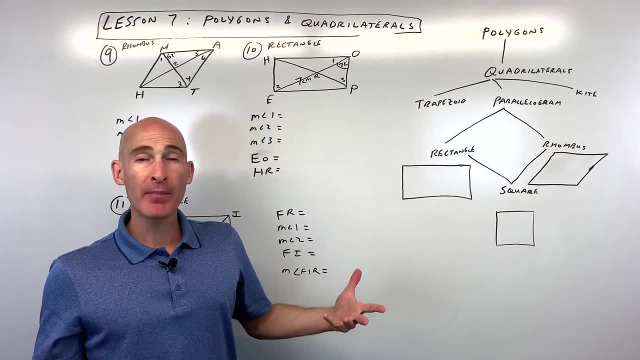 of opposite sides, parallel and congruent. That was this last one here that I told you. a lot of students sometimes forget, So that would be your final step here and you got it. Okay, so we've talked about parallelograms and quadrilaterals and polygons. 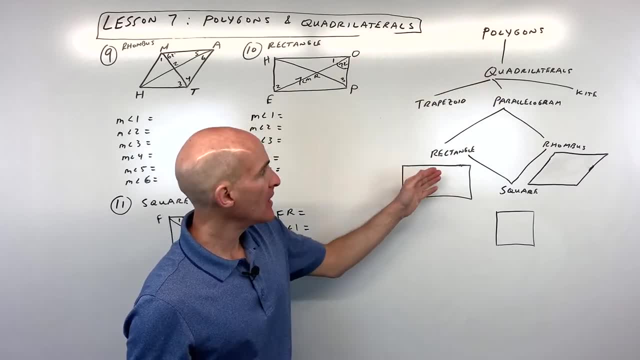 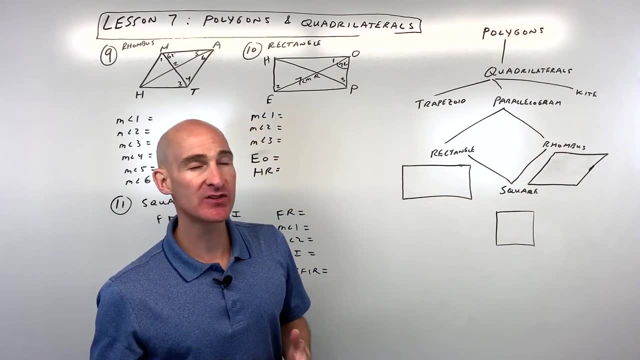 And you can see we're kind of working our way down this tree diagram here. Now we're going to talk about rectangles, rhombi, which is plural for rhombus and square, And we want to talk about their properties. So the nice thing about this tree diagram is: 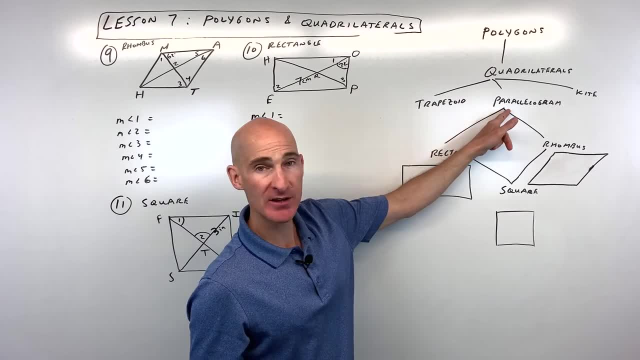 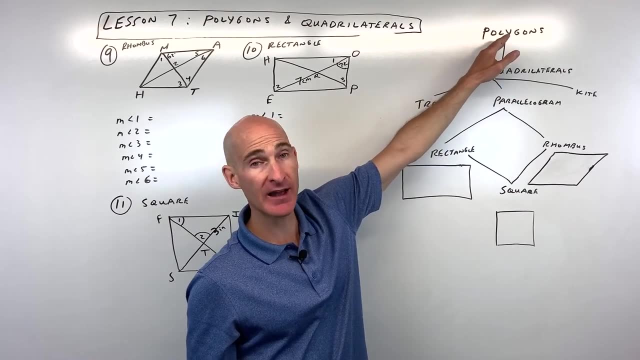 say you're looking at a rectangle. A rectangle has all the properties of a parallelogram- See it's below it on the tree- as well as all the properties of a quadrilateral, as well as all the poly, all the properties of a polygon right. 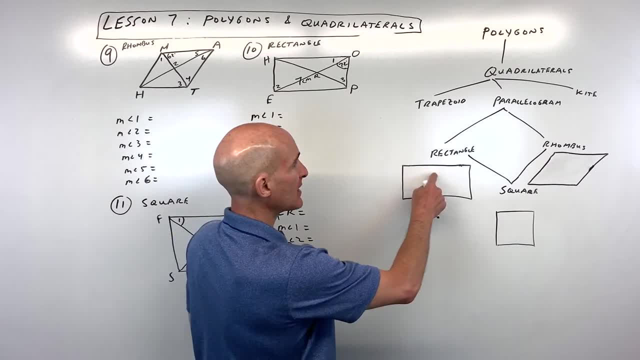 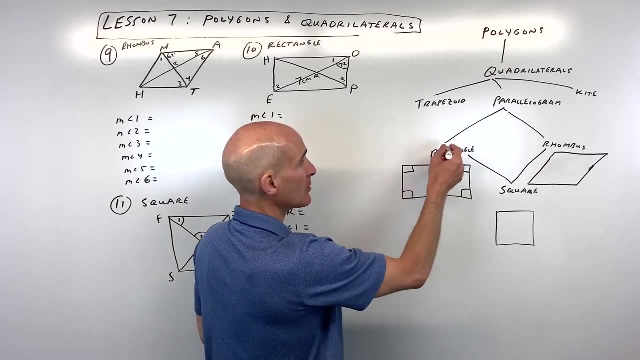 But it has additional properties as well. So, for example, a rectangle is a parallelogram with the addition of having four right angles. So that's what a rectangle is: a parallelogram with four right angles. Not every parallelogram has four right angles, right. 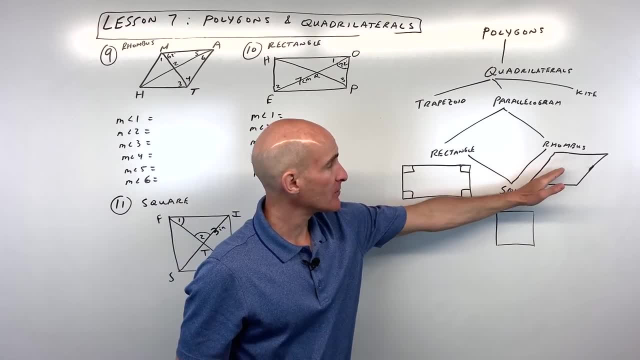 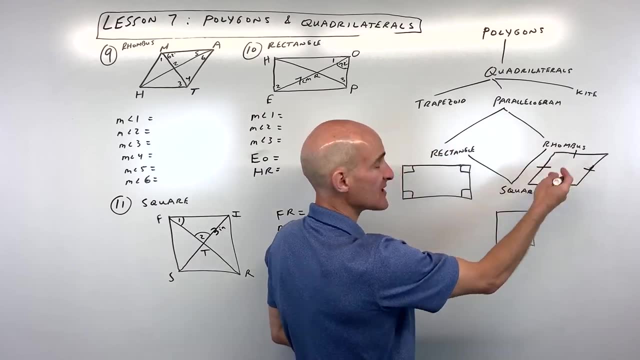 Just a rectangle. Now, what about for a rhombus? Well, a rhombus is a parallelogram, but in addition to all those properties, it has four congruent sides. So all the sides are the same length. And what a square is. 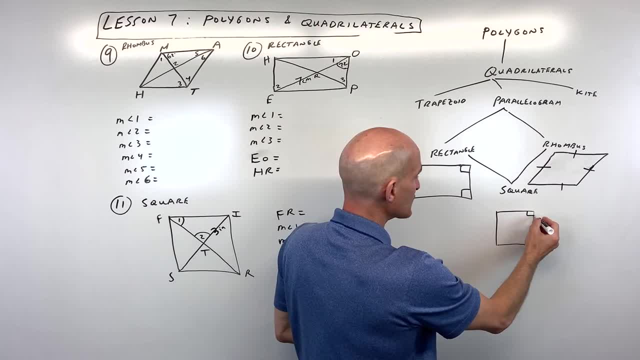 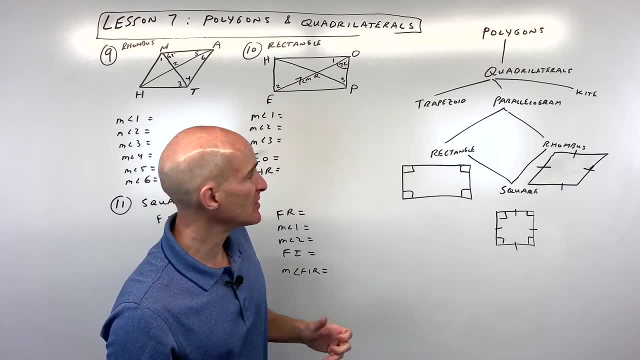 it's a combination of a rhombus and a rectangle. together It has four right angles and it has four congruent sides, But there's additional properties. So let's talk about some of the additional properties. So, if you know, you have a rectangle. 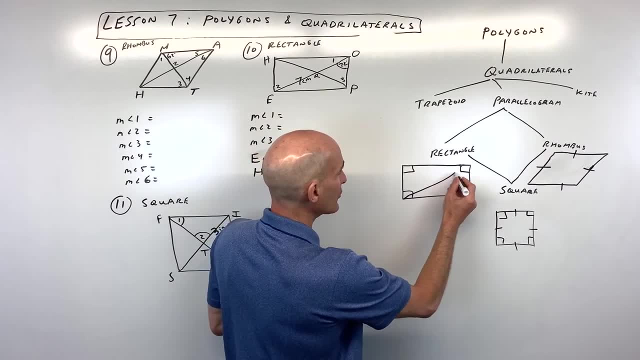 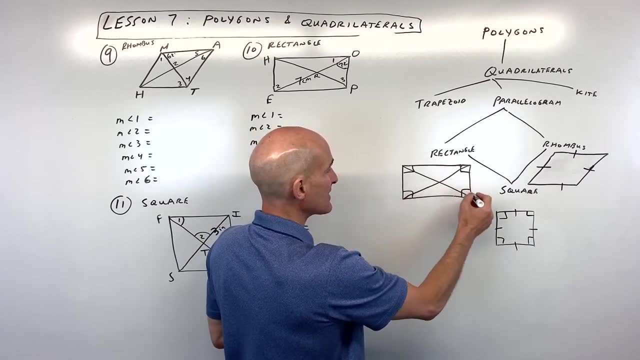 you know you have those four right angles, but when you look at the diagonals, okay, these diagonals, here the diagonals are the same length, So this whole length is the same as that whole length And remember, because it's a parallelogram, the diagonals. 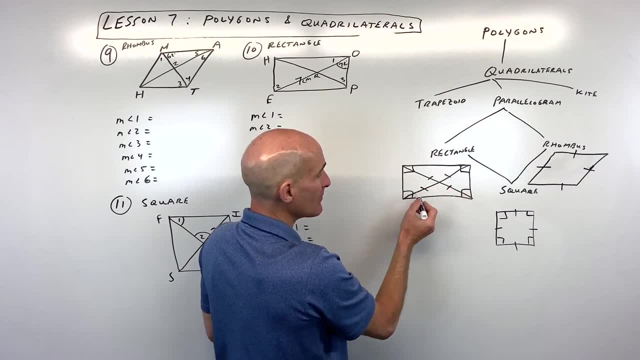 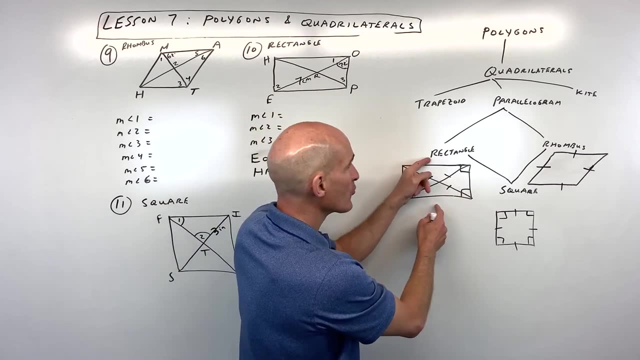 bisect each other. So it works out that all four of these segments are congruent. So the diagonals are congruent and these four individual segments are congruent. Of course, you know the opposite sides are congruent because it's a parallelogram. 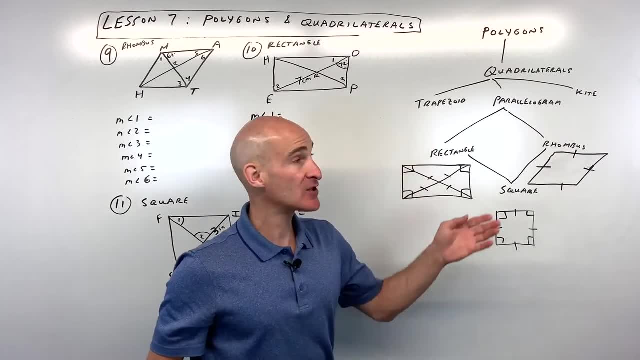 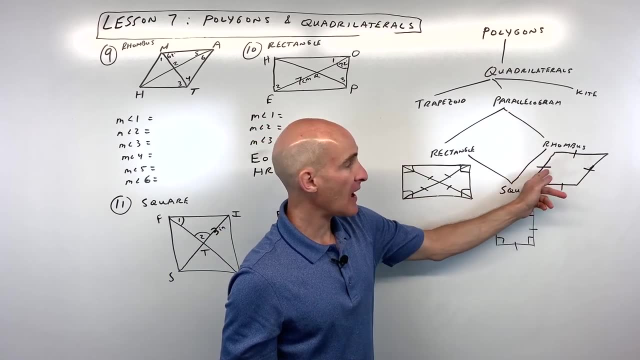 The opposite angles are congruent. The opposite sides are parallel. You know it has all these properties, plus these additional ones here. For a rhombus, though, we said it's a parallelogram with the addition of having exactly all four sides congruent. 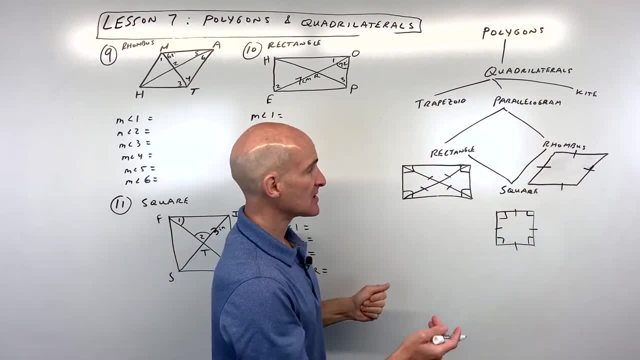 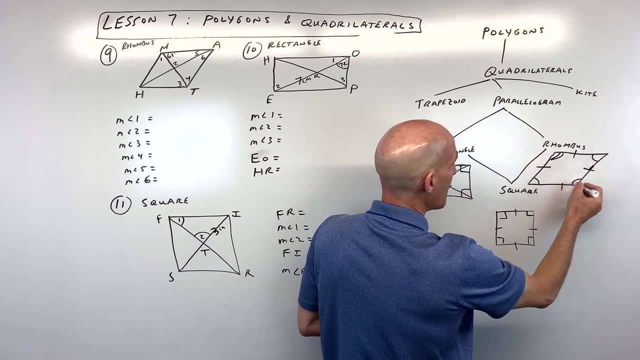 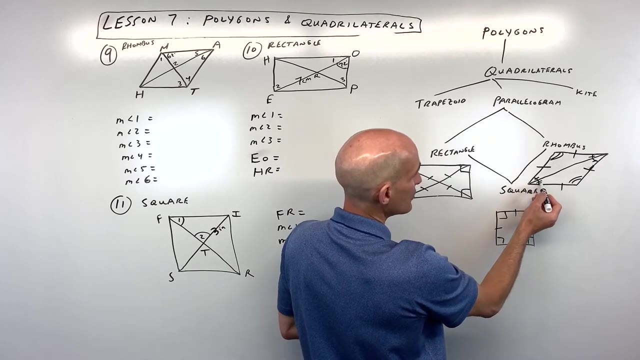 Notice, not every parallelogram has all sides congruent, So that's a special case. So the opposite diagonals. okay, what happens these diagonals? they bisect or cut in half the opposite angles. So you can see that these are congruent. 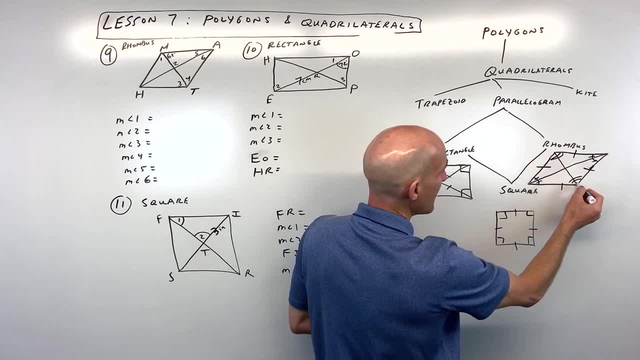 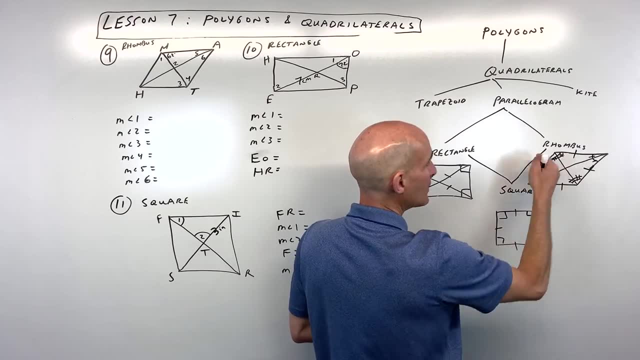 These are congruent. So actually all four of these angles are congruent. And then this diagonal here bisects these guys. okay, So all four of these are congruent. So the diagonals bisect the opposite angles And the diagonals are perpendicular. 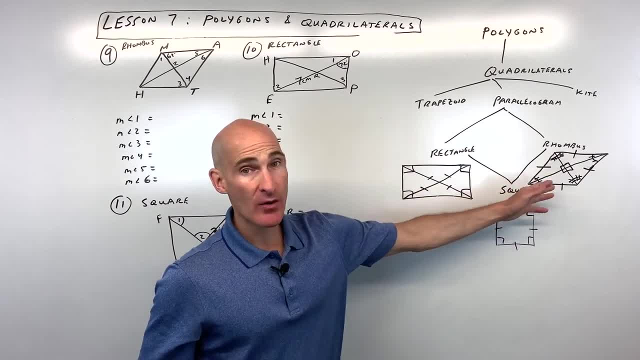 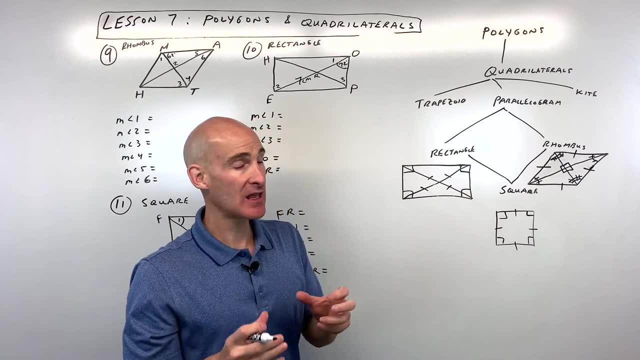 meaning they form, you know, four right angles. So rhombus has got a lot of properties to it Over here. notice the diagonals in a rectangle. These don't form right angles, Okay, so you got to kind of keep these separate. 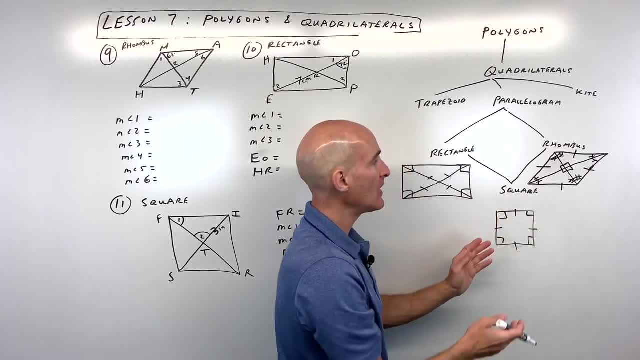 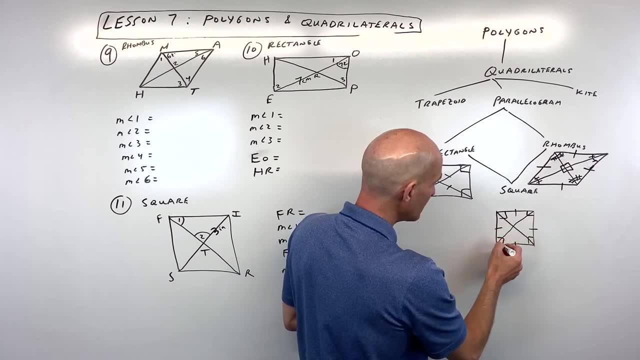 Now a square, because it's a combination of a rhombus and a rectangle. it has all of these properties. So, for example, the diagonals are going to bisect the opposite angles, right Like that. Also, the diagonals are going to be perpendicular. 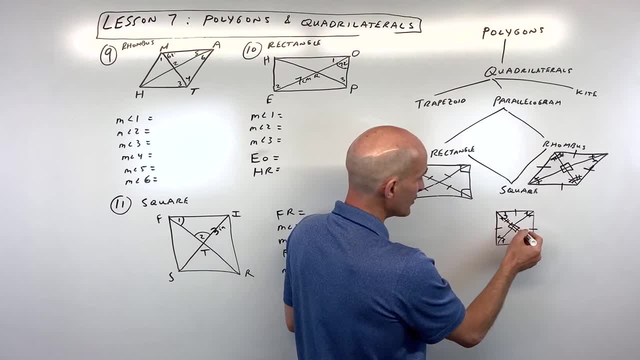 You know the diagonals are going to be the same length because it's a rectangle, then all these are going to be the same. You know it has basically all the properties. So let's look at some examples. So, starting with a rhombus, 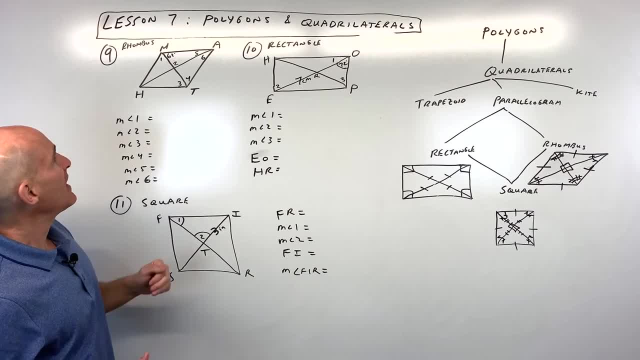 This is rhombus m-a-t-h, right, Rhombus math, okay, And we want to figure out what are the measures of these six angles. So see, if you can do this one, What do you think the measure of angle one would be? 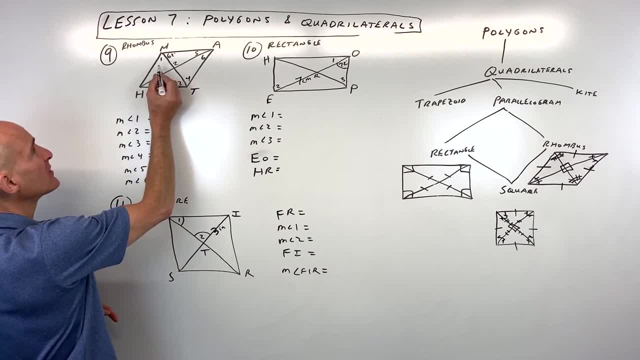 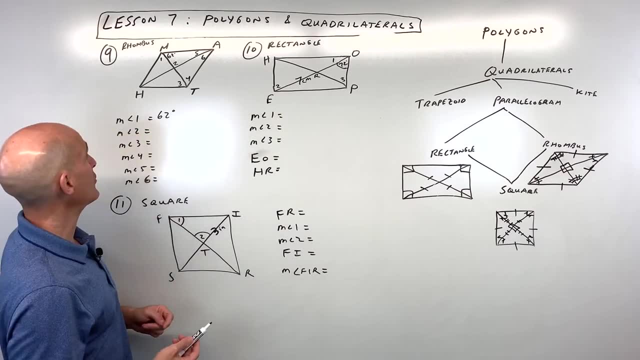 Well, this is 62. We automatically know that this angle is 62, right, Because, remember, we said that the diagonals in a rhombus, they bisect the opposite angles. How about for the measure of angle two? What do you think for that one? 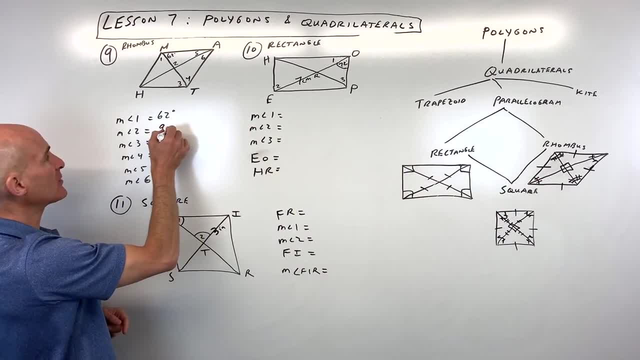 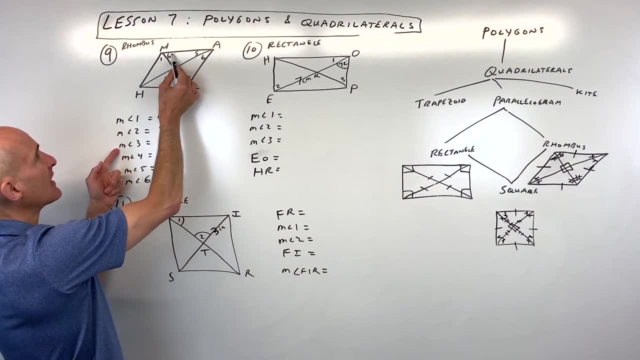 Well, remember, in a rhombus, we said that the diagonals are perpendicular. Perpendicular means that's going to be 90 degree angle. How about for angle three? Well remember, we said the diagonals, they bisect the opposite angles. and we said all. 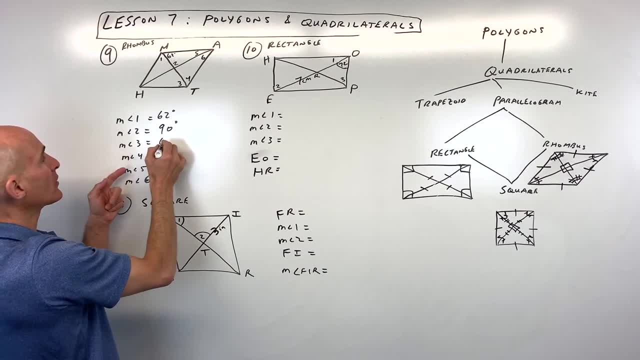 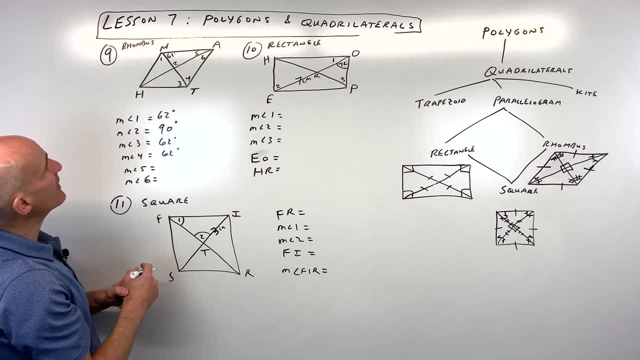 four of these are going to be the same. So angle three, four and one are all going to be 62 degrees. How about for five and six? Okay, now, this is a little bit different here now. So remember we said that this was a right angle: 90.. 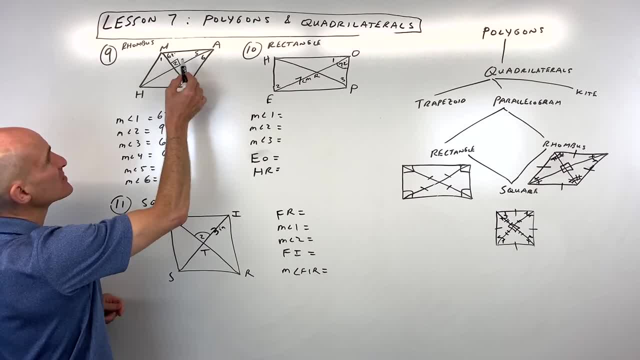 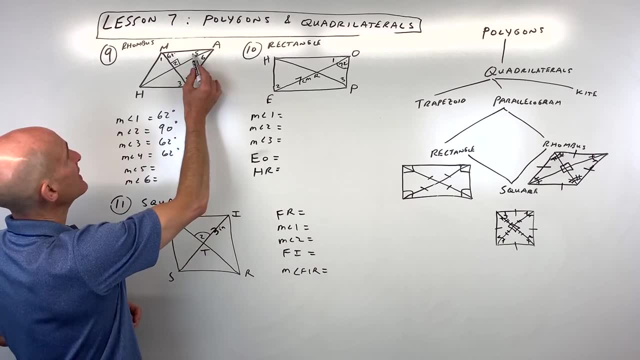 This is 62. So 90 plus 62 is 62.. 62 plus angle five have to add up to 180, because in a triangle all the angles are going to add up to 180. So that means that this is going to be- let's see- a 28 degree angle, right. 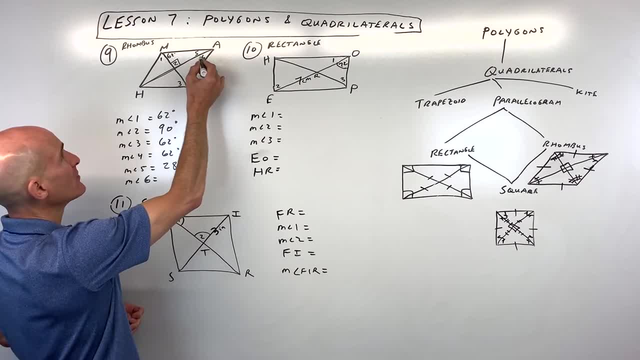 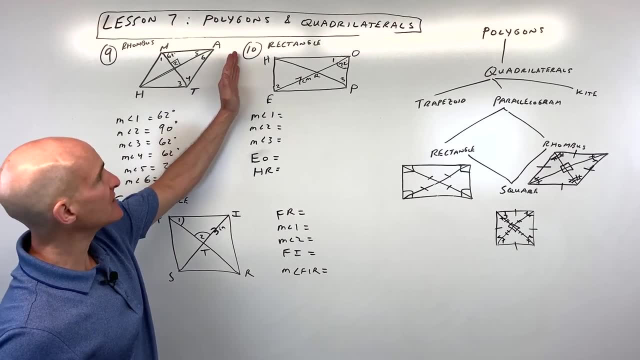 And remember, this diagonal here bisects the opposite angle. So both of these angles are going to be congruent. So that means angle six is also 28.. Okay, so let's see if we can do number 10 now. Number 10, we have a rectangle, rectangle hope- H-O-P-E and the diagonals they bisect. 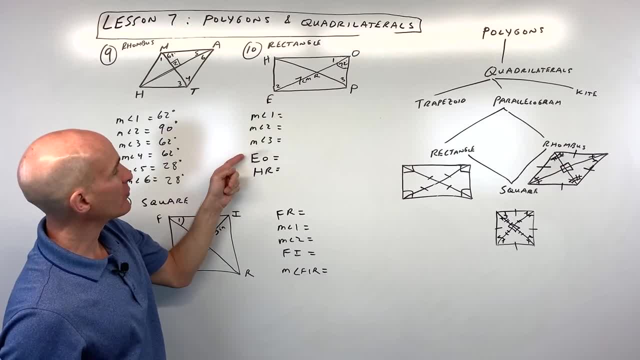 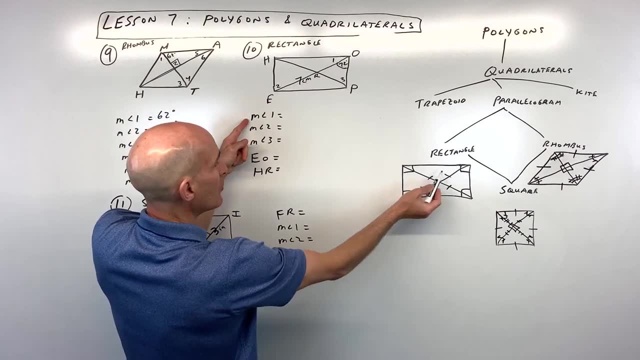 at this point. here are, And we want to find, the measures of angle one, two, three, the length of E-O and H-R. See if you can do that one. Well, the measure of angle one, let's see. remember, in a rectangle we have four right. 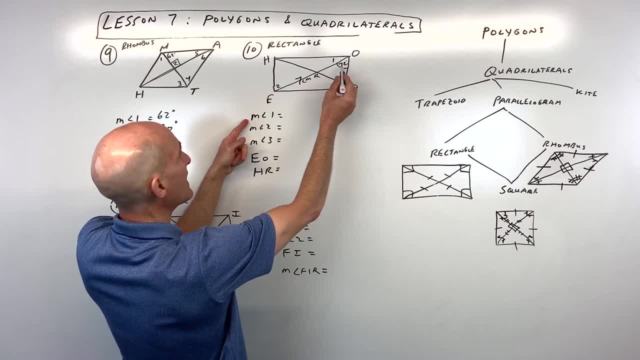 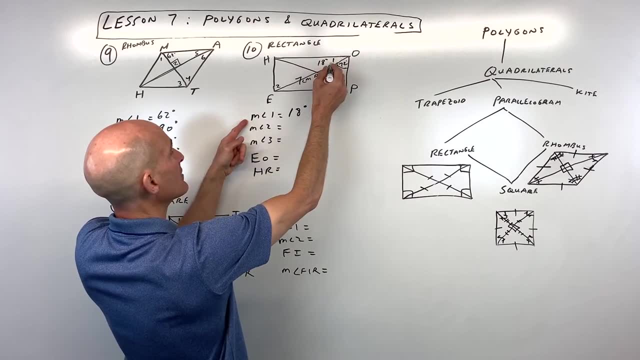 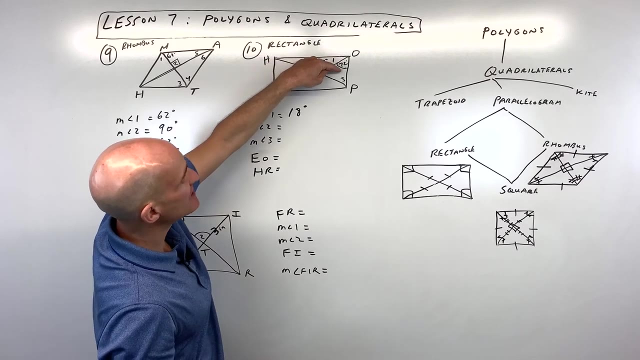 angles. So if this is 72, that means that this must be 90 minus 72 or 18 degrees. Sometimes I like to write right on the diagram because I might need that later in the problem. Okay, measure of angle two. let's see this. angle here should really be the same as this. 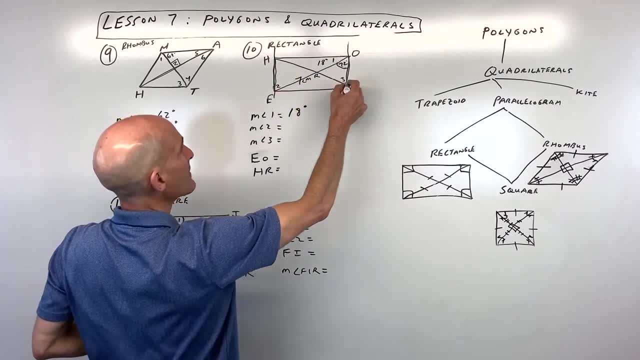 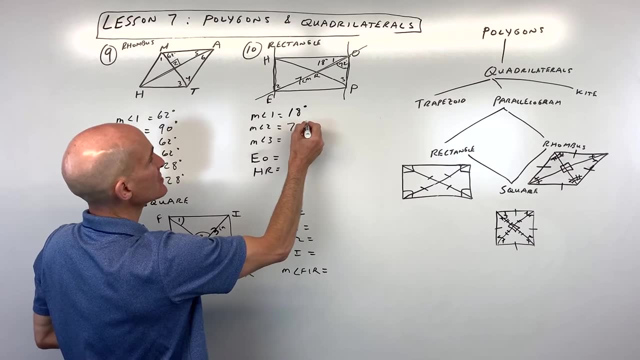 angle here. Why is that? Well, because, remember, it's a parallelogram. the opposite sides are parallel. This is like a transversal. these are actually alternate interior angles. So that means angle two is 72.. How about the measure of angle three? 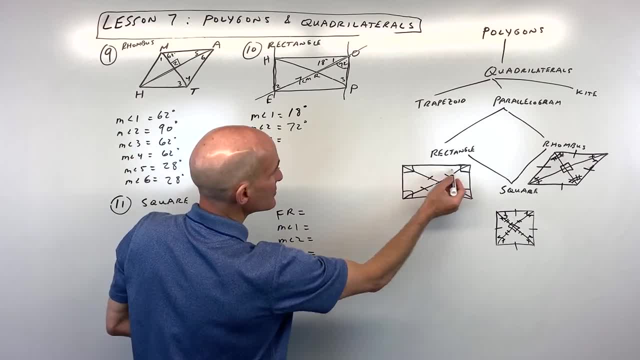 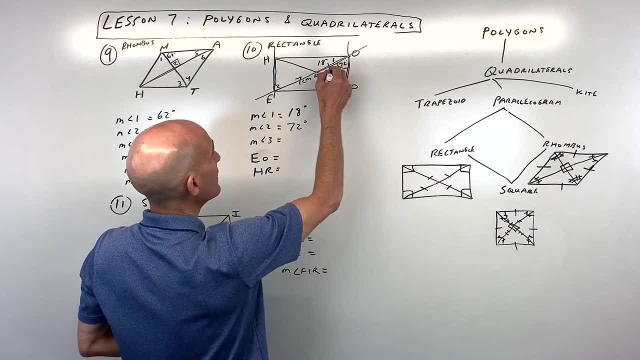 Okay, this is an interesting one, because remember how we said that the diagonals they're the same length, And because it's a parallelogram, the diagonals bisect each other. so all four of these pieces are the same. Well, if these two sides are congruent, what kind of a triangle has two sides congruent? 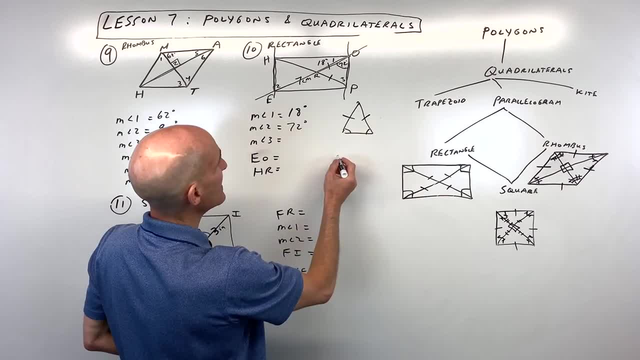 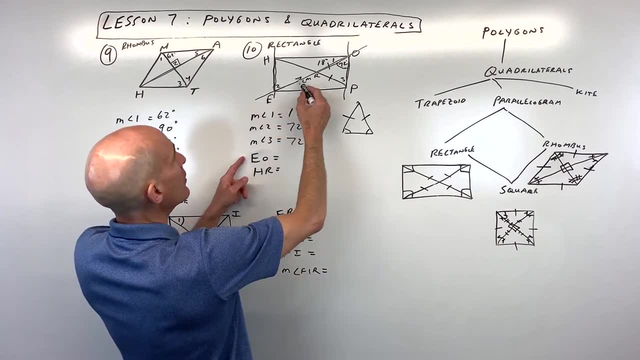 An isosceles triangle right. And what do we know about the base angles of an isosceles triangle? They're congruent. so that means angle three is 72 as well. And then let's see the length of EO, that's this whole diagonal. 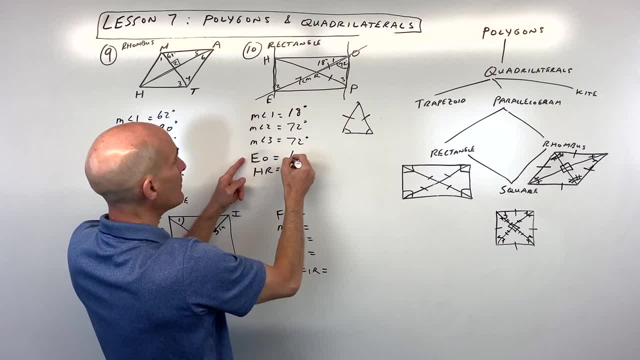 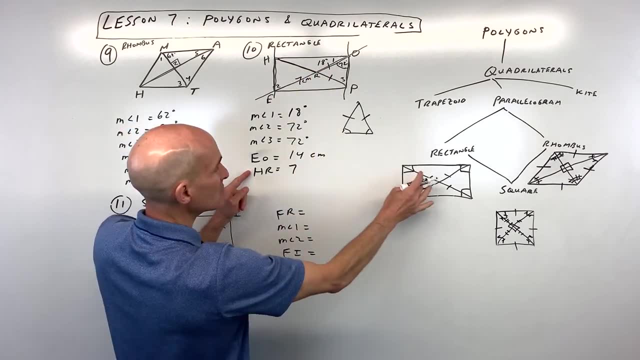 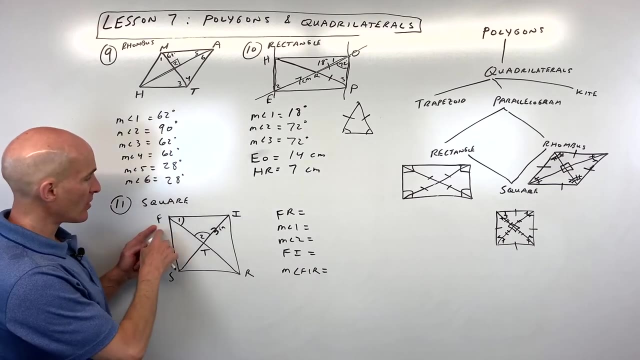 Well, if ER is seven, EO must be double 14 centimeters and HR, which is this length here, must be the same length as ER. that's also seven, because we said all four of these are congruent. Okay, so that's a rectangle. now for this one. here we're talking about a square, square. 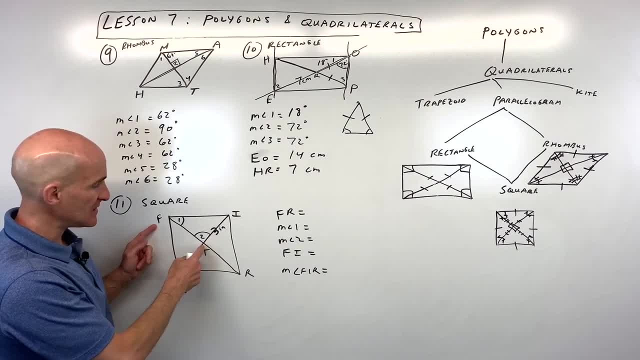 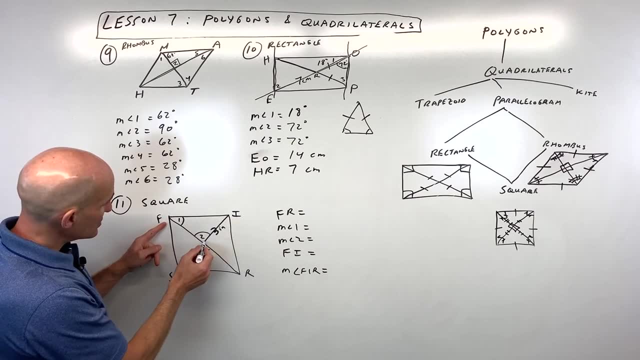 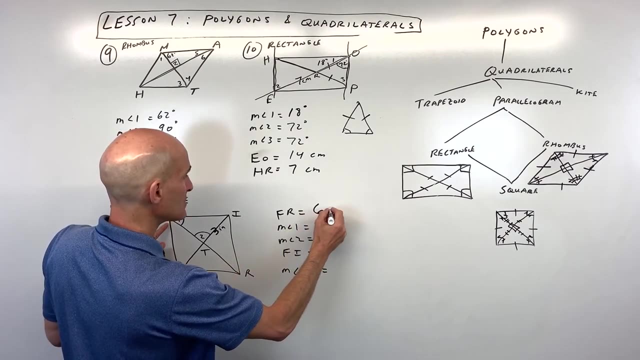 FIRS And the diagonals cross at T, so this is FIRST, Let's see. so what's the length of FR? Well, if this is three inches, that means this is three, this is three, this is three. so from F to R, that's three plus three, which would be six inches. 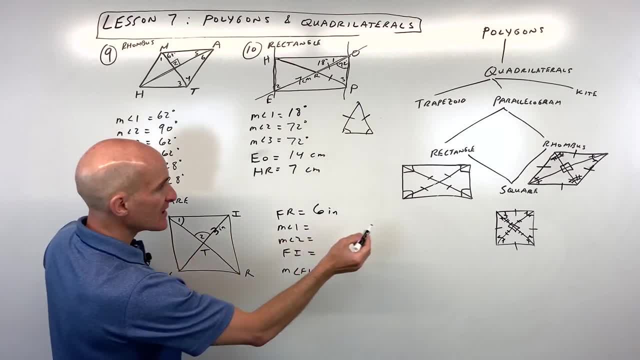 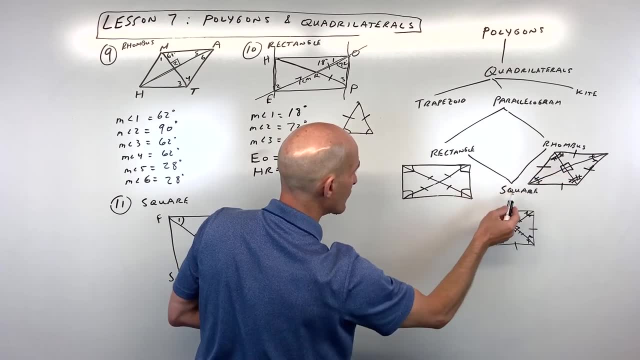 How about the measure of angle one? Well, remember, we said: in a square, this is a special type of rectangle, right, All the angles are 90 degree angles and we know the diagonals. in a rhombus they bisect. 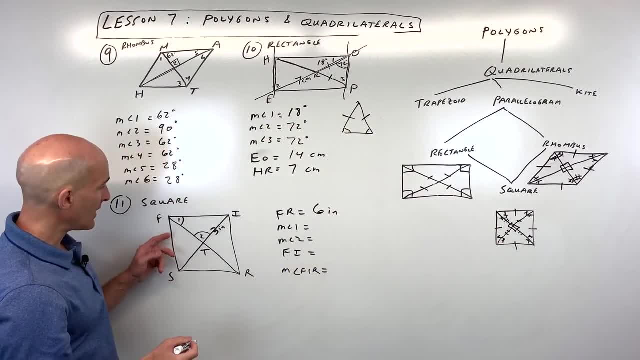 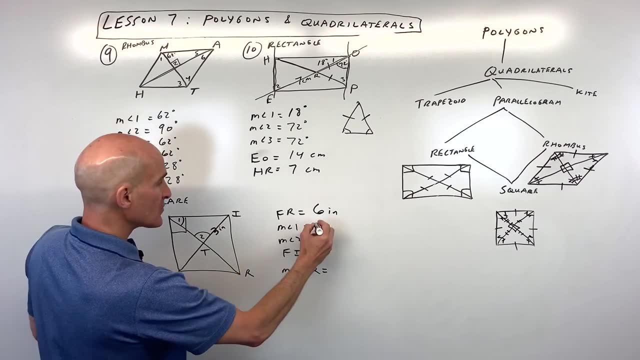 each other. So the combination of square is a combination of a rectangle and a rhombus. that means that this angle, this angle, are both going to be 45, because, remember, this was 90 and it's bisected. So angle one is 45 degrees. okay, how about for measure of angle two? 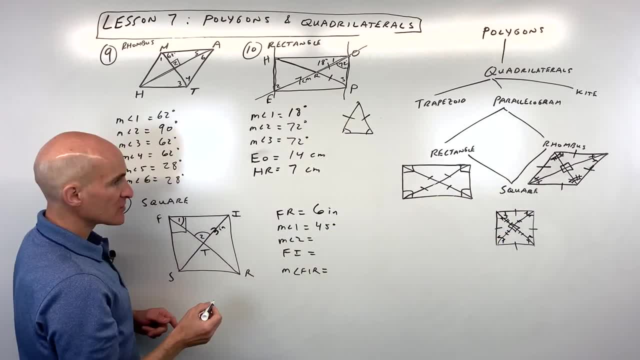 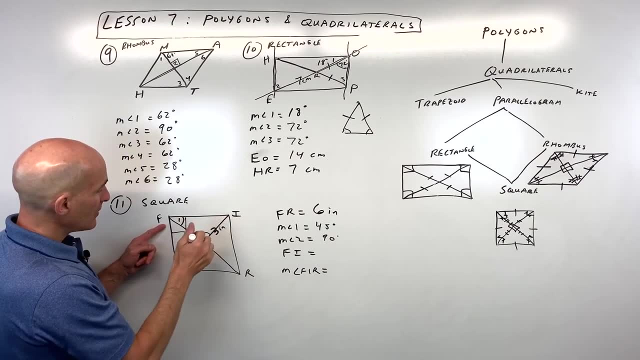 Well, remember the diagonals in a rhombus, they're perpendicular, and a square is a special type of rhombus, so that's going to be a 90 degree angle. Okay, how about the length of FI right here? Well, if this is 45,, and this is 45, and this is 90,, right? 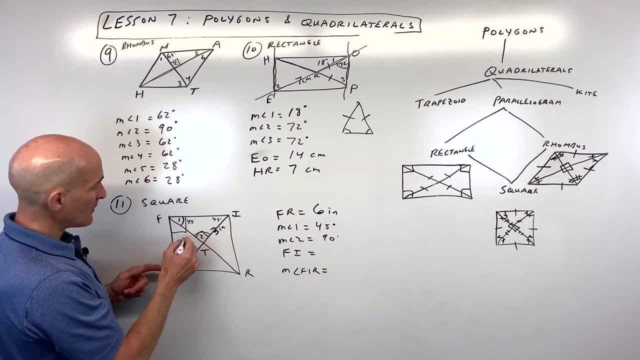 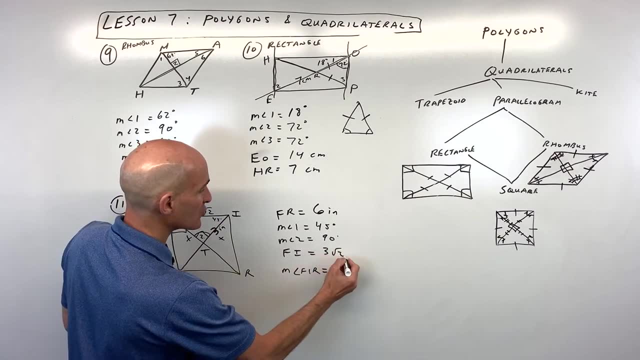 That's a special right triangle. it's a 45,, 45,, 90.. That means, whatever this side is, x, x, x, root two. so if this is three, this must be three times the square root of two. that's from our special right triangles. 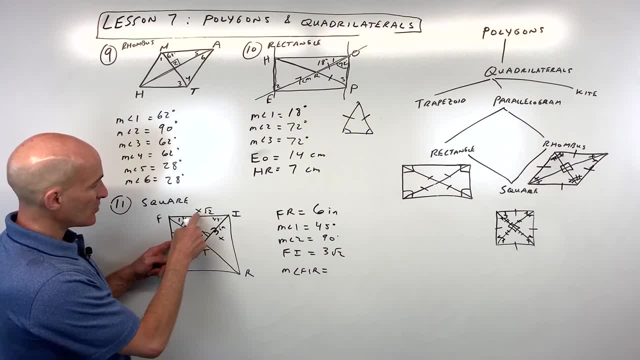 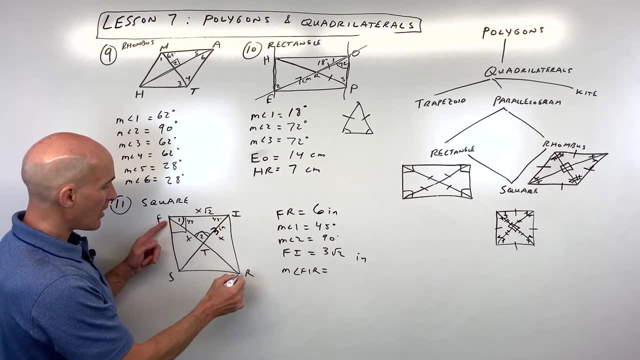 You could also do Pythagorean theorem: if this is three, and this is three, you could do: a squared plus b squared equals c squared and solve and that's going to be inches. And then the last one, the measure of angle: FIR F-I-R. that means this would also be: 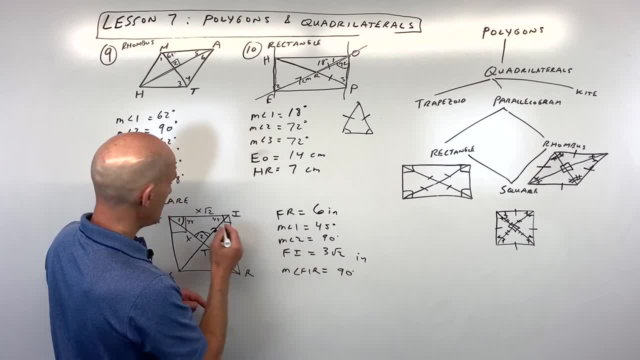 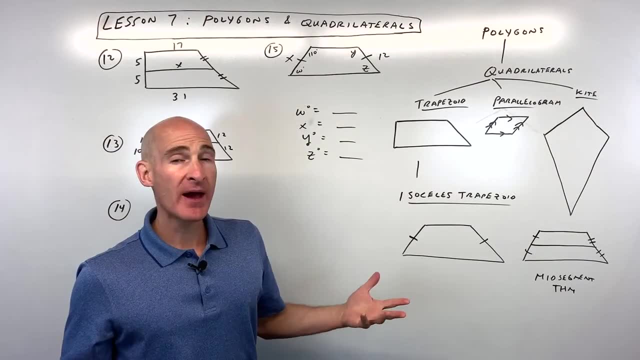 a right angle be 90 degrees, because all the angles in a rhombus are 90 degrees, Okay, And a rectangle are right angles and a square is a special type of rectangle. Okay, let's go back to our polygon tree diagram again, and here we talked about polygons. we 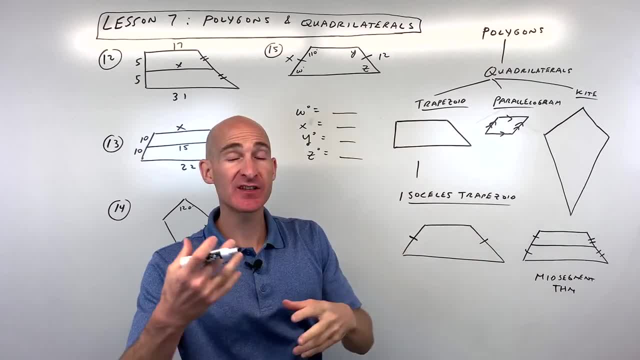 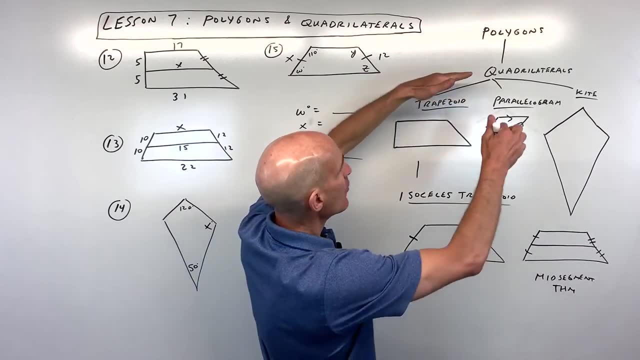 talked about quadrilaterals. we talked about parallelograms and then the special types of parallelograms like the rectangle, rhombus and square. But going back up to quadrilateral again, what we can do is we can branch out here to 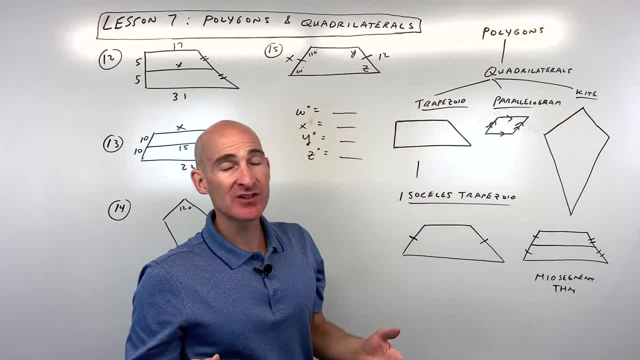 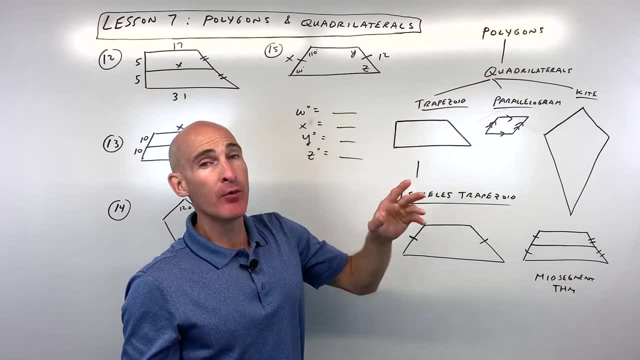 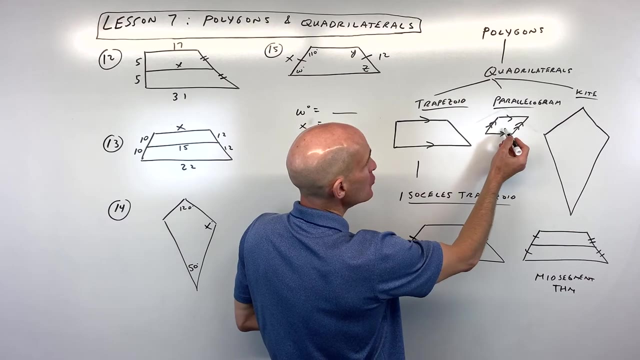 trapezoids and kites. Now, what exactly is a trapezoid and a kite, Excuse me? Well, a trapezoid it's a quadrilateral meaning. it has four sides, but what it does is it has one pair of opposite sides, parallel, whereas, remember, in a parallelogram you had two pairs. 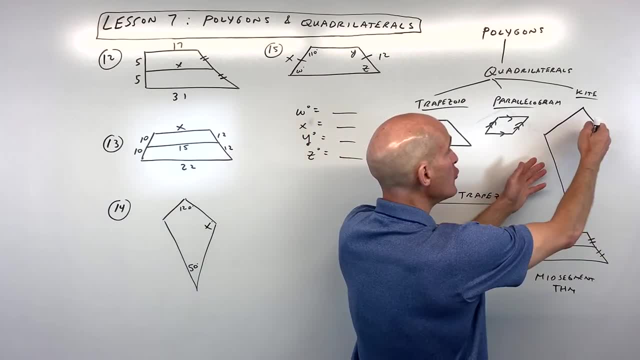 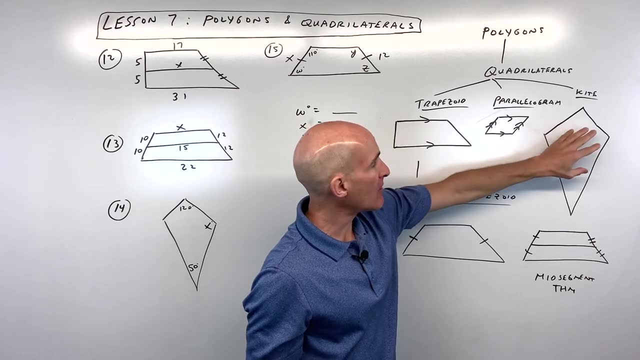 of opposite sides parallel, and in a kite you have no pairs of opposite sides parallel. So that's kind of one way of distinguishing. you know, do you have a parallelogram, a trapezoid or a kite? But when you talk about a kite, okay, the opposite sides are not parallel, but what's? 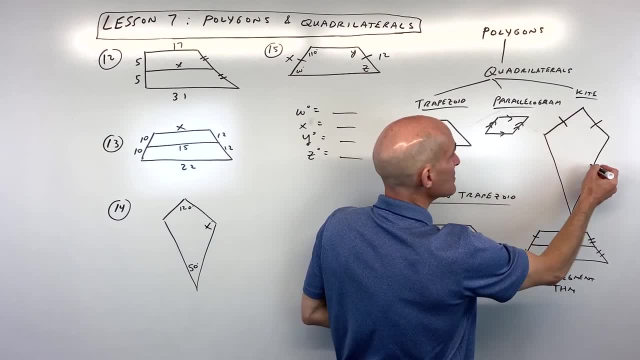 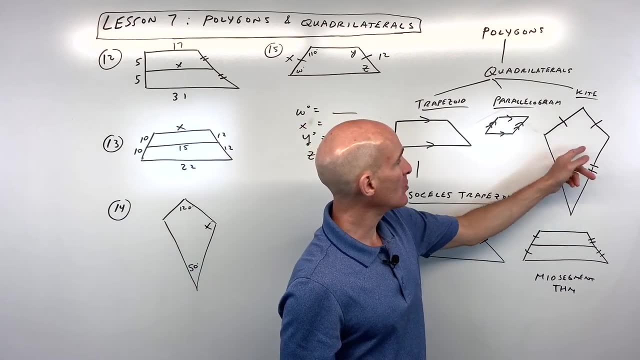 interesting about a kite is it has two pairs of kites. Okay, They're consecutive sides. congruent Consecutive means like one after another, like these ones that are next to each other. These are congruent. That's a pair. These are congruent. 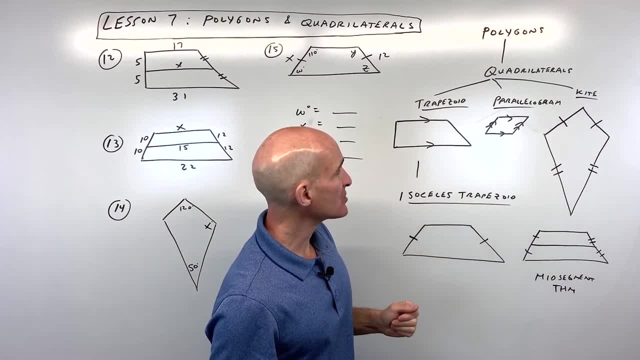 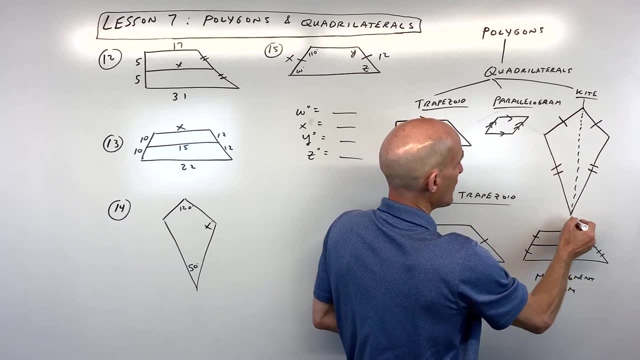 These ones here are not congruent. Now there's more properties to kites. What you can think about with a kite is you can think of this as like a line of symmetry, Okay, And what I mean by that is, if you fold it over this line, everything that matches up. 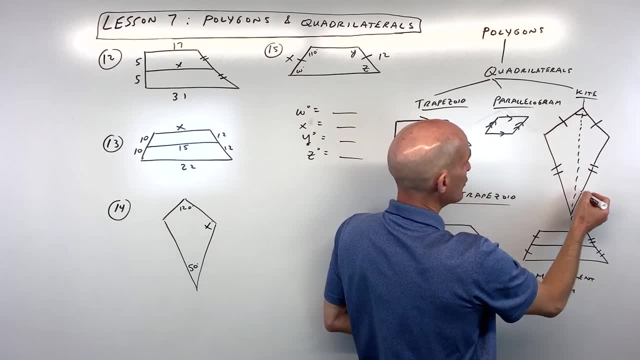 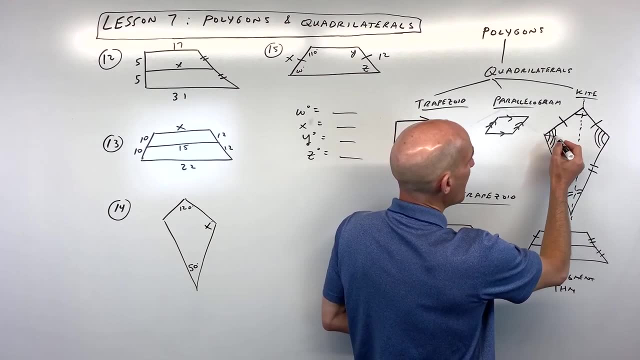 will be congruent. So, for example, like this angle and this angle will be congruent, this angle and this angle will be congruent, This angle here and this whole angle here will be congruent. And then when you draw the diagonals, okay, the diagonals, this, of course, will be the 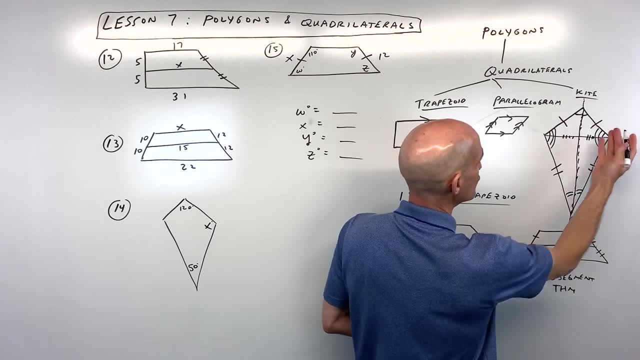 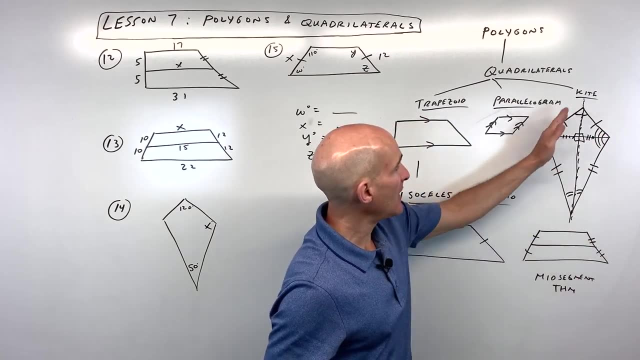 same as this. okay, because we said this was like a line of symmetry. you can fold it this way, but not this way. right, The diagonals are going to be perpendicular. they form those four right angles. So a kite. just remember that line of symmetry, that will really help. and it has two pairs. 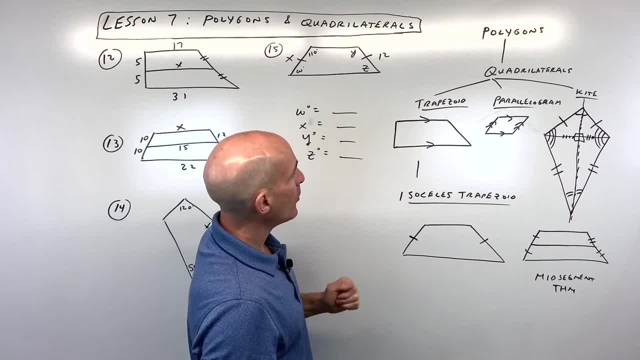 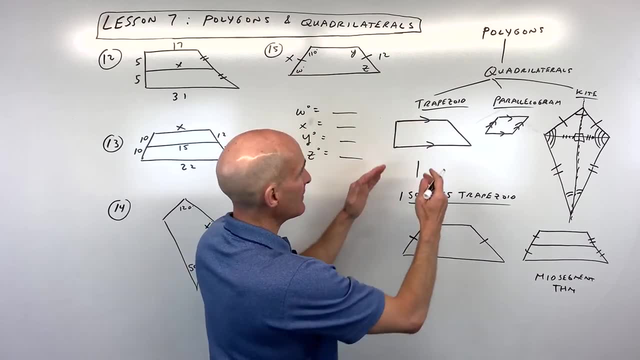 of consecutive sides congruent With a trapezoid. though let's talk about a trapezoid. these sides that are parallel, right, These are what are referred to as the bases, okay, And then these sides are referred to as the legs or the sides. 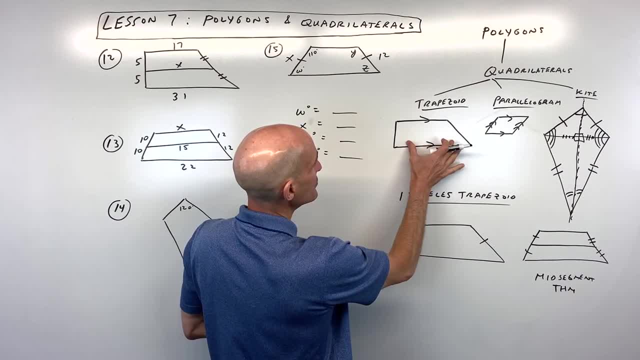 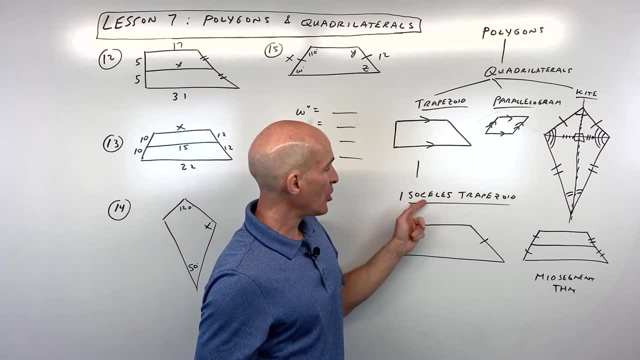 These angles here are what are called base angles. This is a pair of base angles and these two here at the top. that's called a pair of base angles. So in a trapezoid there's a special type of trapezoid called an isosceles trapezoid. 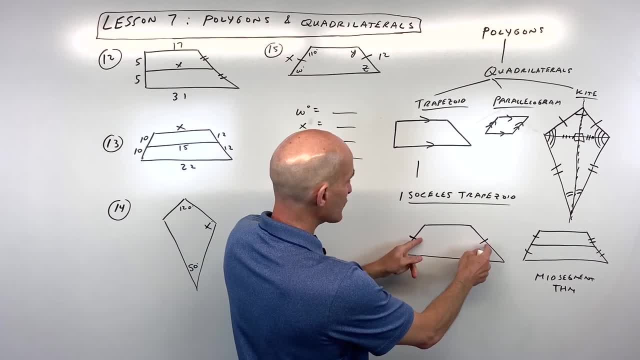 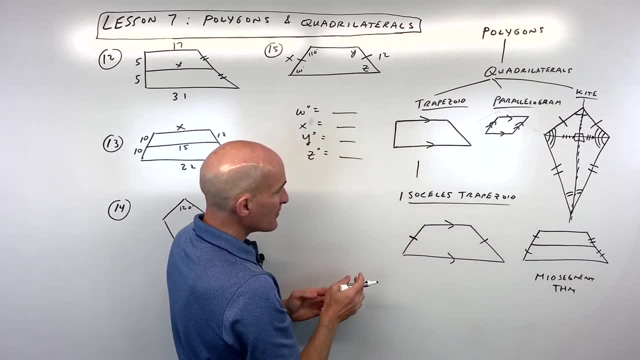 kind of like an isosceles triangle, where the two legs or the two sides are congruent. So these are the same here. you can see these are not the same. These are parallel. But there's more interesting properties with isosceles trapezoid, because what happens is: 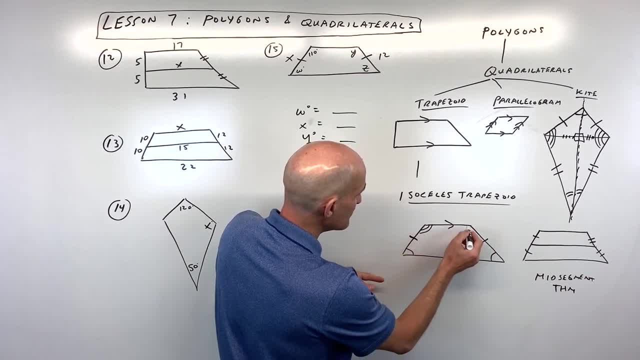 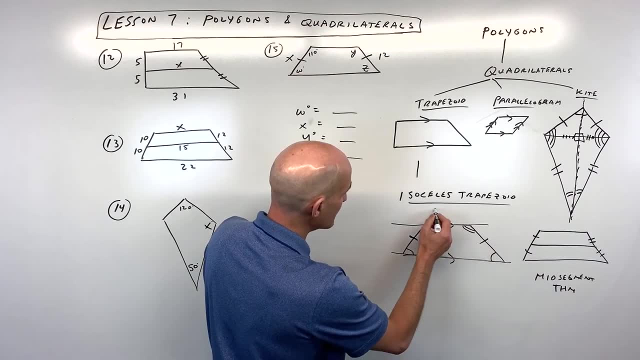 the base angles. these are congruent. and then these base angles are congruent, whereas these two angles are actually supplementary because, remember, this is a parallel line, this is a parallel line, this is a transversal. These are like consecutive interior angles, they're supplementary. 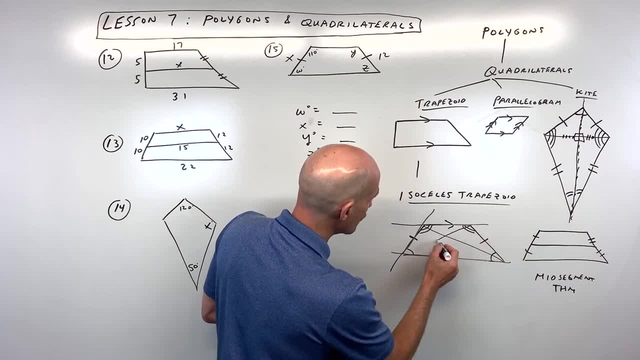 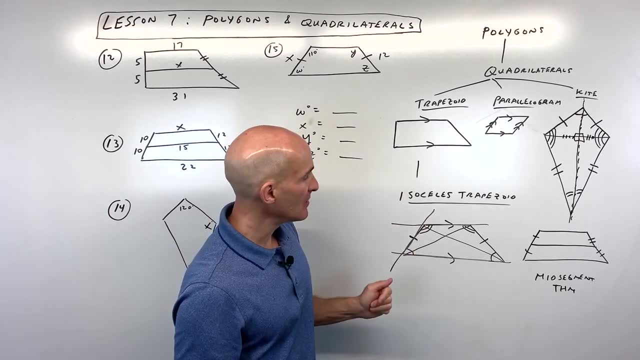 Also for isosceles trapezoid. the diagonals are congruent, they're the same length, but they don't bisect each other. they don't cut each other in half like they did in a parallelogram. Okay, so basically, we've got our trapezoid, we've got our kite. 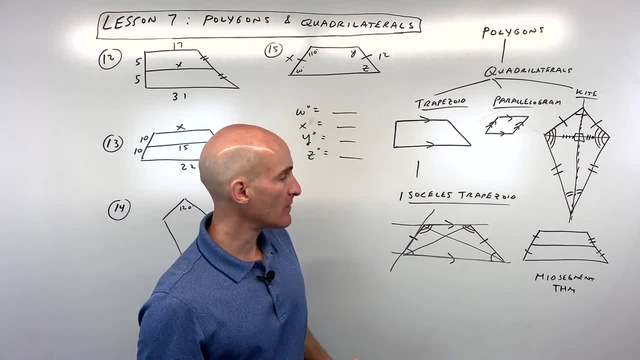 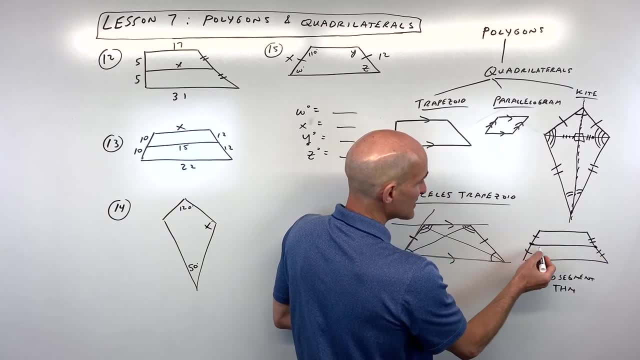 The other thing we want to talk about with trapezoids is what's called the mid-segment theorem, and what the mid-segment theorem is is, when you draw this line that connects the two midpoints of the legs or the sides, see how it's cutting this side in half. this 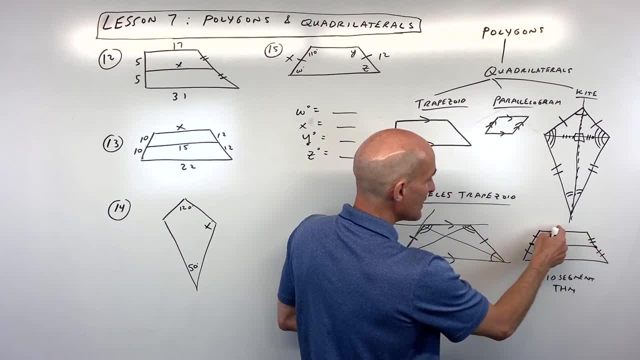 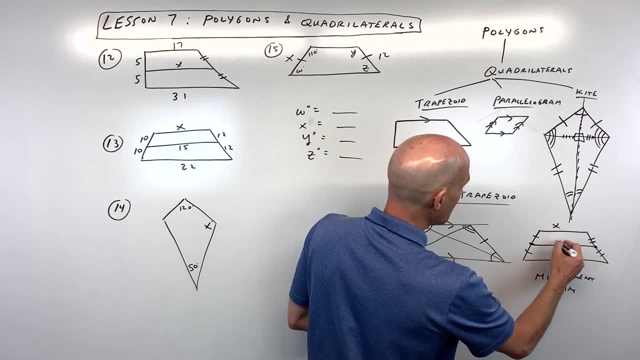 side in half. the length of this mid-segment is going to be the average of the two bases. So what do we do when we find an average? Well say, for example, this was like x and this is y, and the mid-segment length was z. 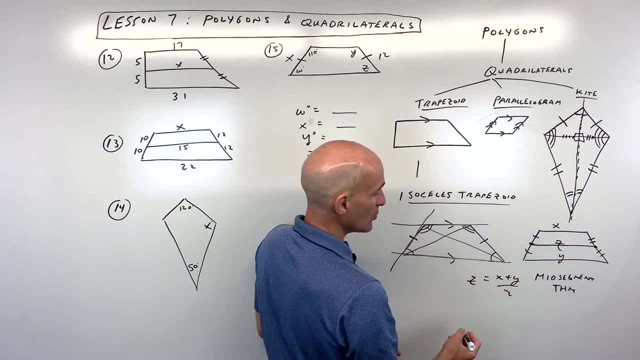 You would say that z equals x plus y, Y divided by 2.. So it's like if this was 80 and this was 100, you'd say 180 divided by 2 would be 90.. So that's the mid-segment theorem. 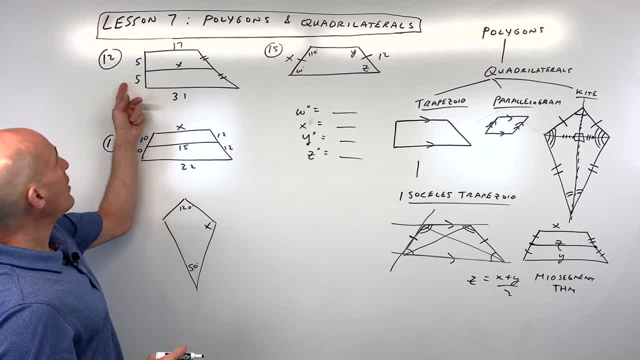 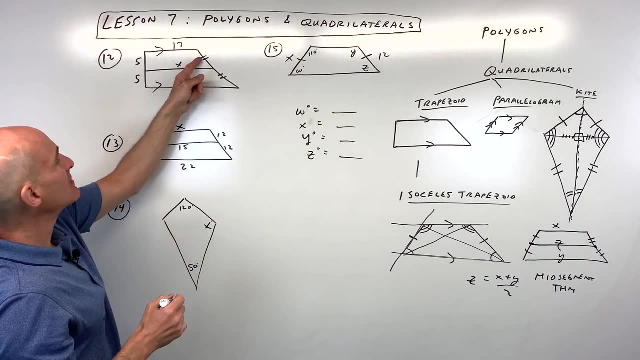 So let's see if we can try some problems now. So for number 12, you can see we have a trapezoid, okay, and you can see this is 5 and this is 5. These are congruent. so it's connecting the two midpoints. so you can see x is a mid-segment. 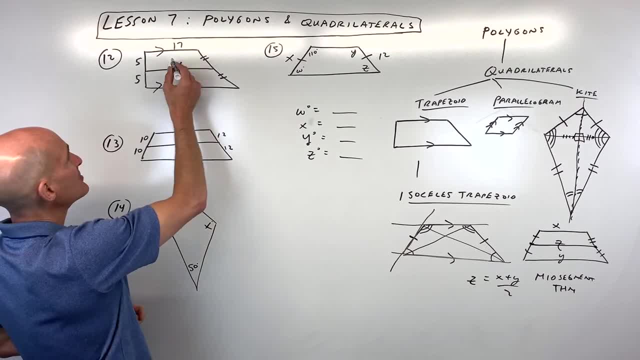 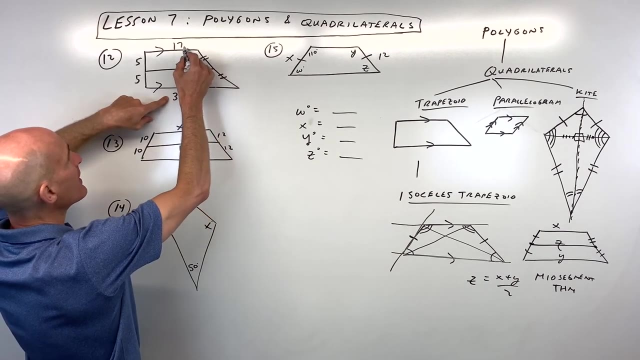 So how do we find the length of this mid-segment? Well, we can add these together: That's going to be 17 plus 31.. That's 48.. Divided by 2 is going to be 24.. Notice that 31 minus 7 is 24, 24 minus 7 is 17. or you can say: 17 plus 7 is 24, 24 plus 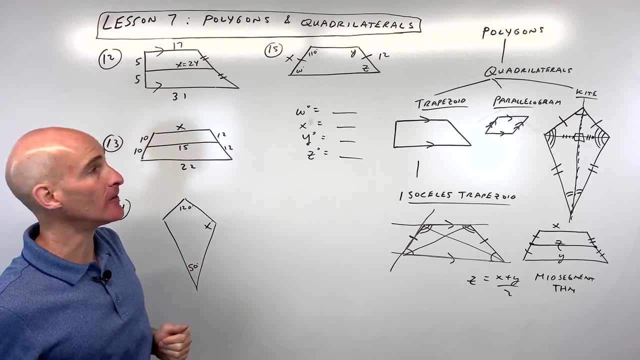 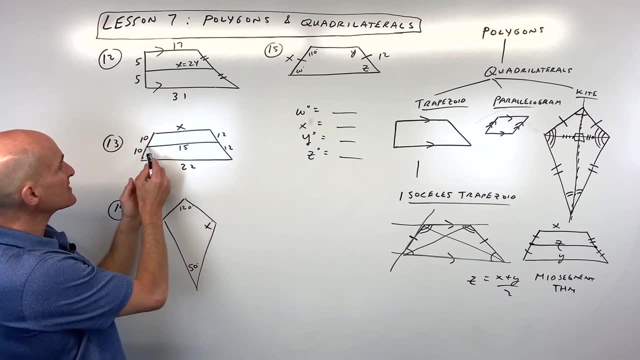 7 is 31.. It's halfway in between right It's in the middle, But I just like to do the average here. So for number 13,, this one's a little bit different. Sometimes this confuses students, because they give you the mid-segment, they give you the. 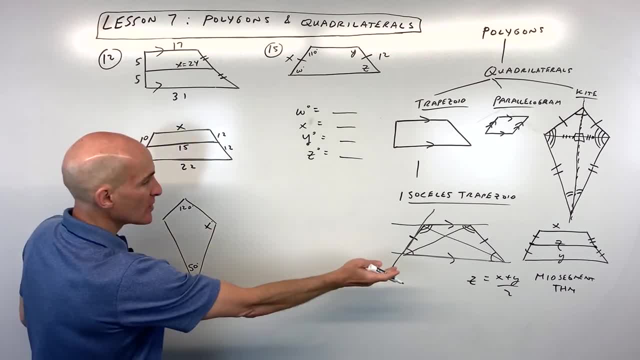 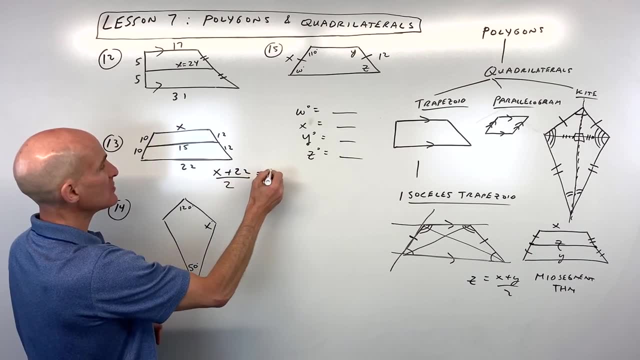 base, but they don't give you the other base Still, though, So we can use this equation, the mid-segment theorem. We can say this base x plus this base 22, divided by 2, is equal to the mid-segment 15.. 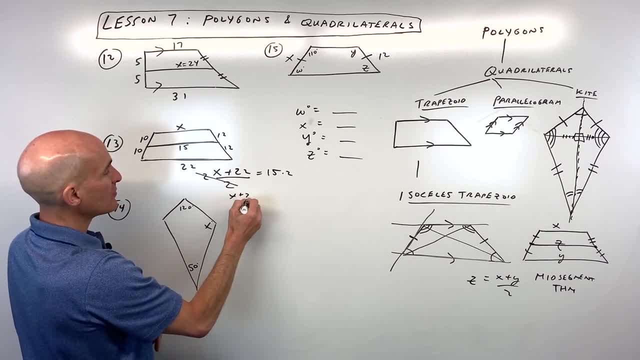 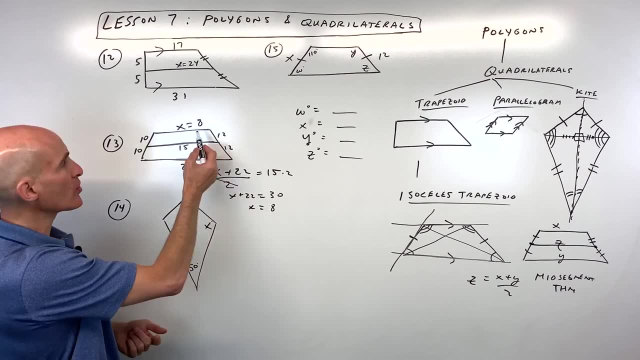 Then we can just multiply both sides by 2. So we have: x plus 22 equals 30. Subtract 22 from both sides and you can see that x must equal 8.. You can check your work: 8 plus 22 is 30, divided by 2 is 15.. 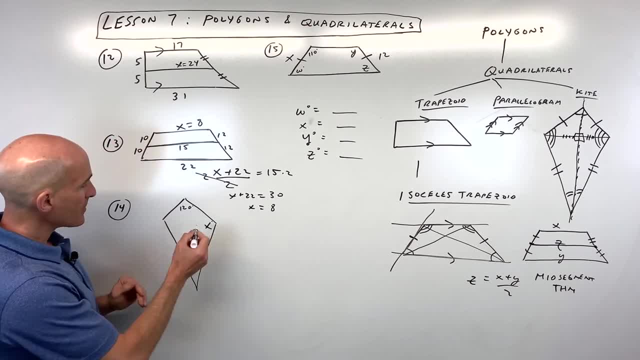 It checks out For number 14. here we're given a kite- Okay, Okay, Right- And we want to find the missing angle measure here. Well, this one's kind of an interesting problem because you can see it's a quadrilateral. 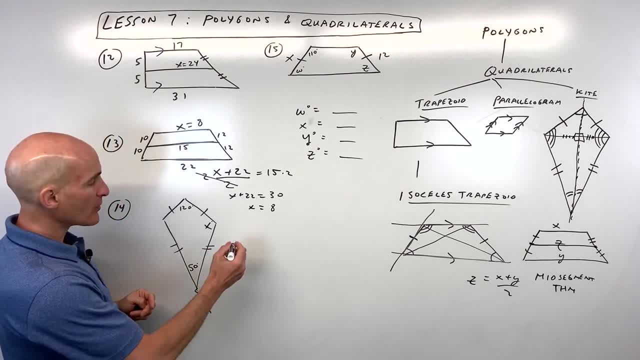 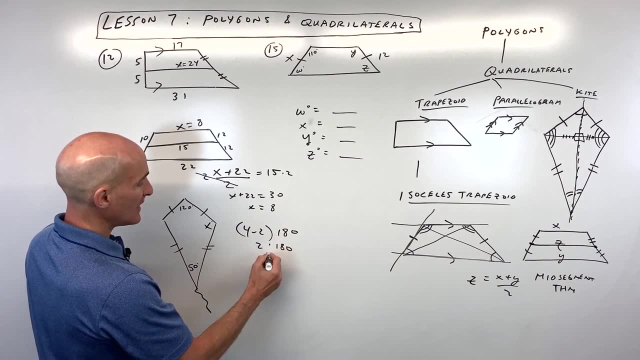 There's four sides, There's four angles, And we know, in a quadrilateral from our polygon, interior angles, theorem n minus 2 times 180.. Two times 180 is 360.. So we know all these angles add up to 360.. 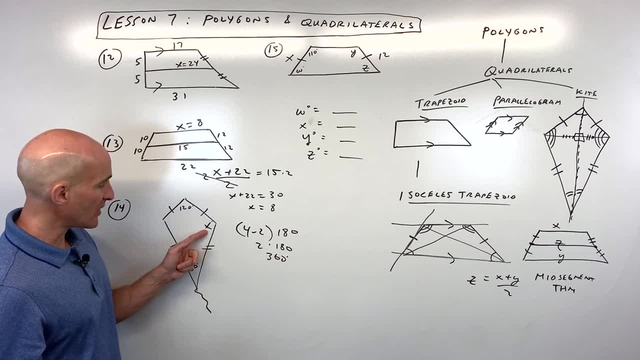 But you can say: well, Mario, we're only given three of the angles and we're trying to find one of them. But remember how we said that With a kite you can fold it over that line of symmetry that goes straight down the middle. 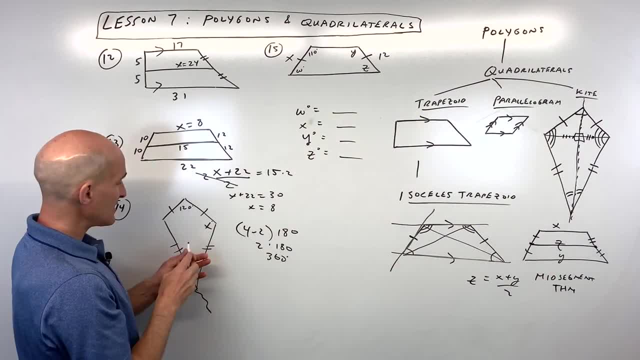 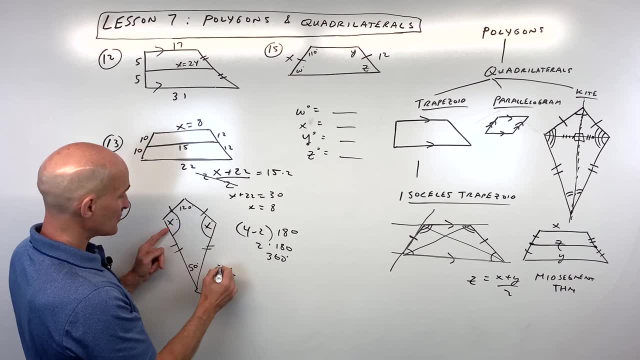 here like that. Okay, So that means if I fold this, this angle here, x is going to be the same angle as this guy over here. So now we can write an equation. We can say x plus x, which is 2x plus 120 plus 150, that's 170.. 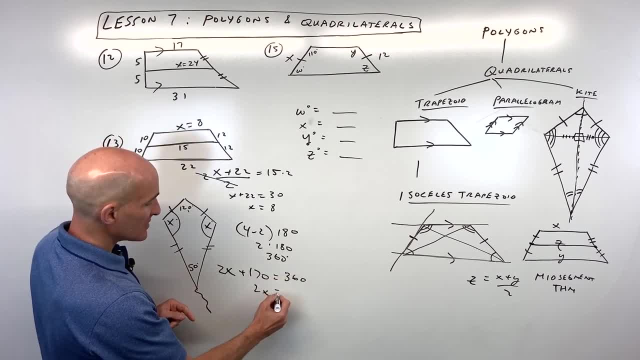 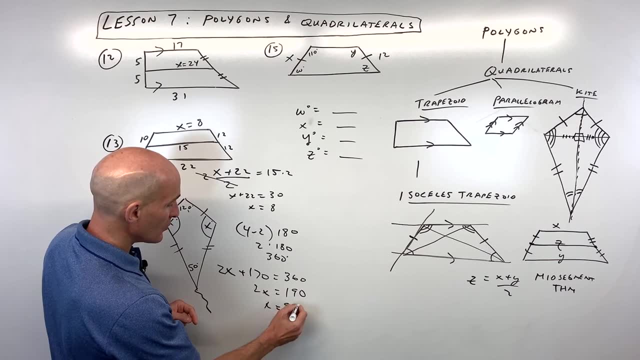 All those angles have to add up to 360.. If we subtract 170 from both sides, we get 190. And if we divide both sides by 2, we get x equals 360.. Okay, So 2x equals 95 degrees. 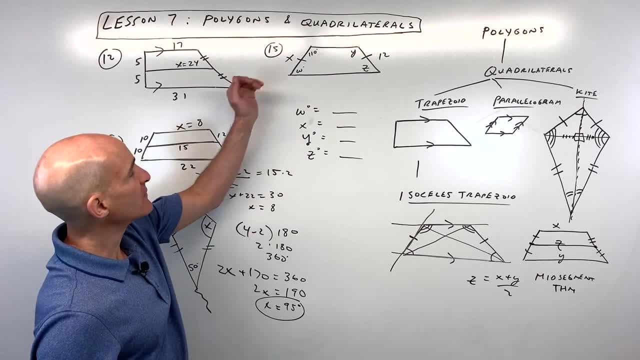 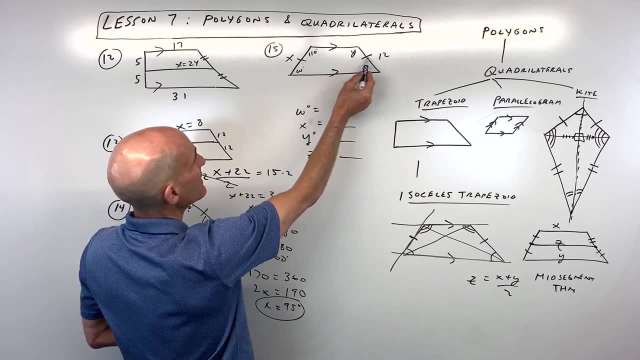 So each of these would be 95.. Okay, And then for number 15, here we're given an isosceles trapezoid. You can see both sides here are congruent, the legs and these are parallel. So how would we solve for w, x, y and z? 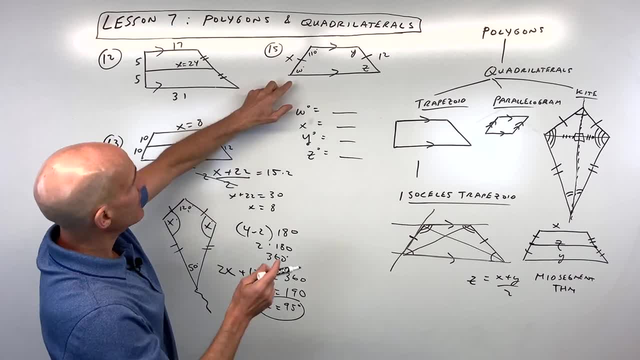 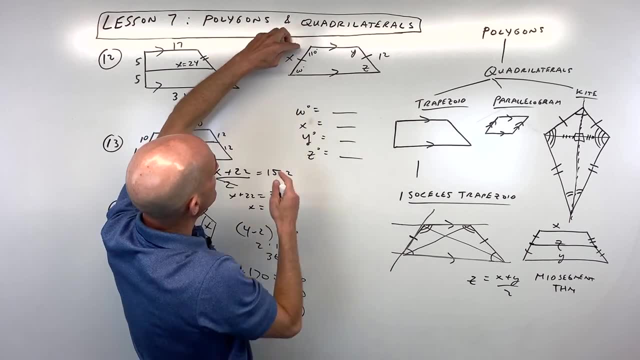 So what do you think for that one? Well, remember that if it's an isosceles trapezoid, the base angles are going to be congruent, So w is going to be the same as z. Oh, That's where w are. 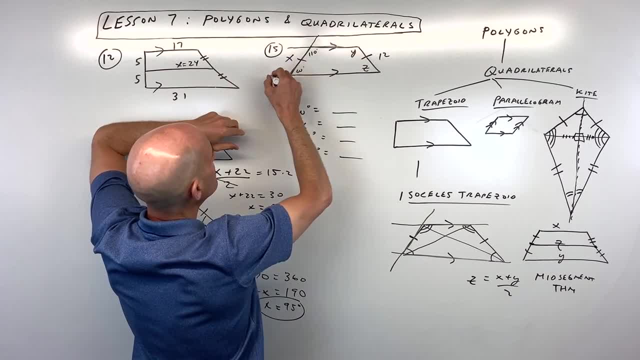 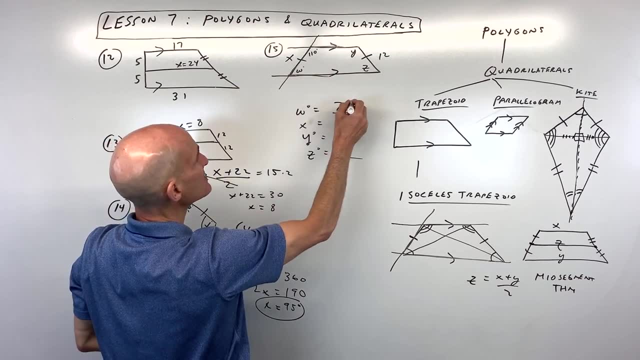 So what about over here? Well, we know that this is a parallel line and this is like cut by a transversal. We know that these angles are going to be consecutive interior angles. they're supplementary. so that means that w must be 70 degrees.